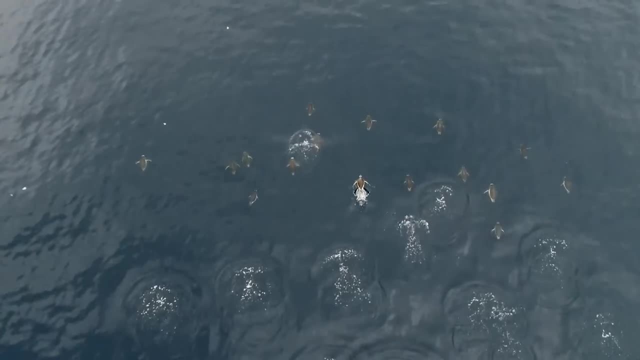 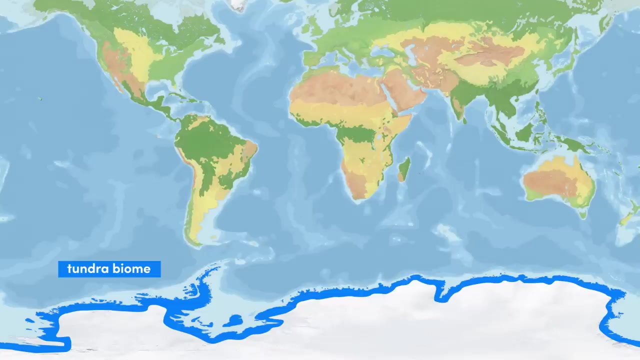 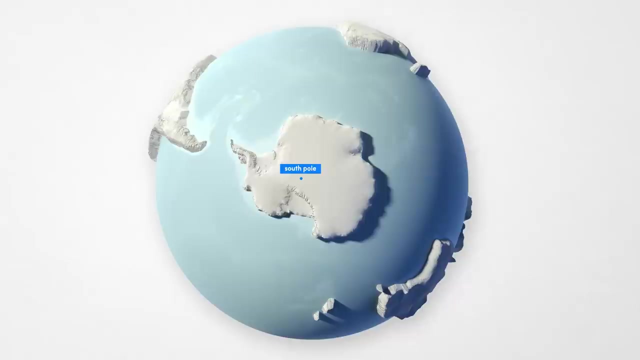 making migration impossible for terrestrial mammals. There are very few animals who can survive the harsh conditions here, and those who do thrive, fly or swim. While its outer ring of tundra is the only biome, the topography and geographic makeup of this realm are interesting, to say the least. The main landmass is split into two parts. 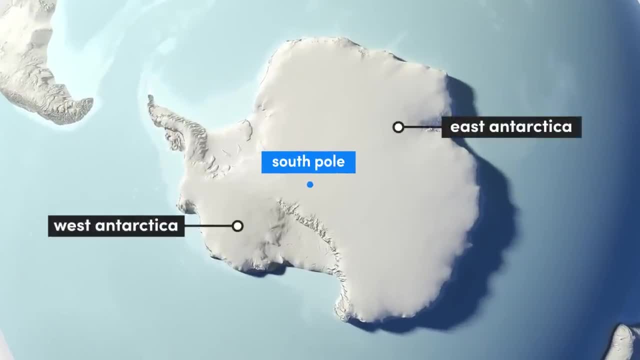 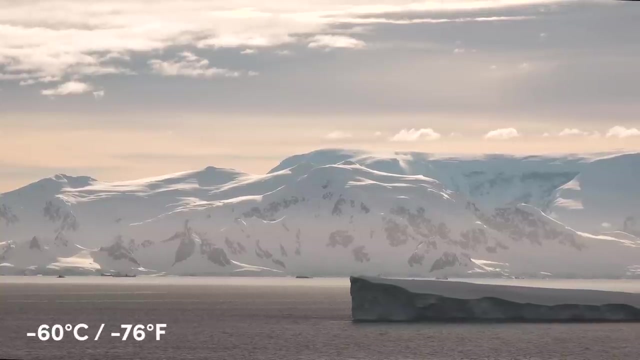 East Antarctica and West Antarctica, which are divided by the Transantarctic Mountains. While a good portion of the east sits over 3,000 meters, its highest peak, Vinson Massif, is found to the west, overlooking the Rhone Ice Shelf, With temperatures reaching as low as 60°C. the top of the mountain is the highest peak. Vinson Massif is found to the west, overlooking the Ron Ice Shelf, While a good portion of the east sits over 3,000 meters. the top of the mountain is the highest peak. 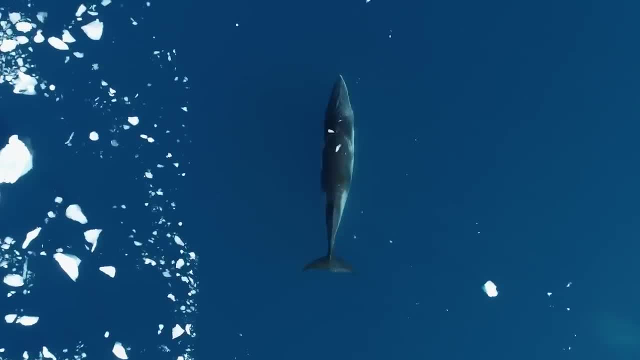 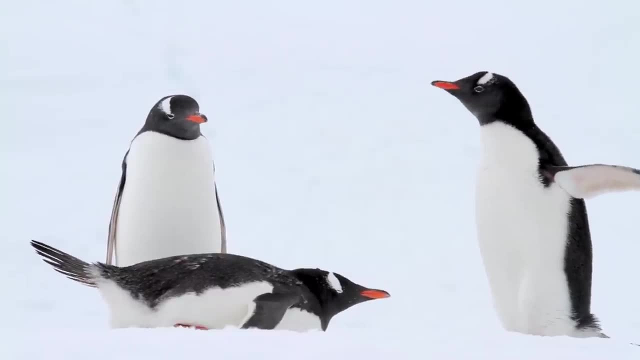 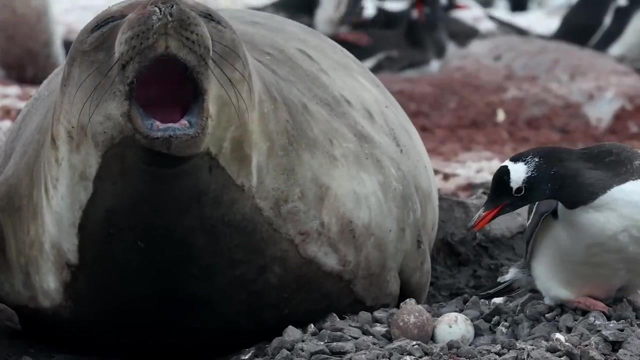 and winds of up to 100 mph. the conditions of this realm are brutal. However, there are a few advantages. For a start, there are no land predators here, no polar bears, no arctic wolves. Combine this with an abundant supply of krill and fish and, for those who can put up with the 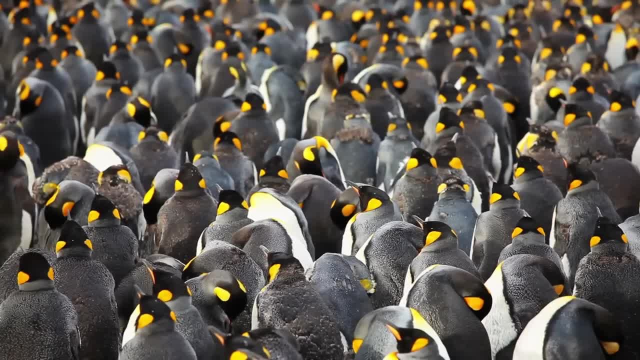 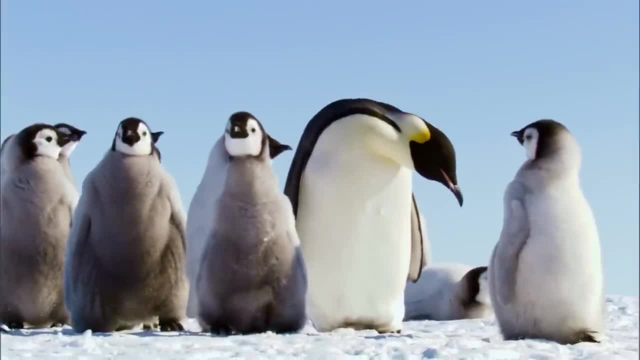 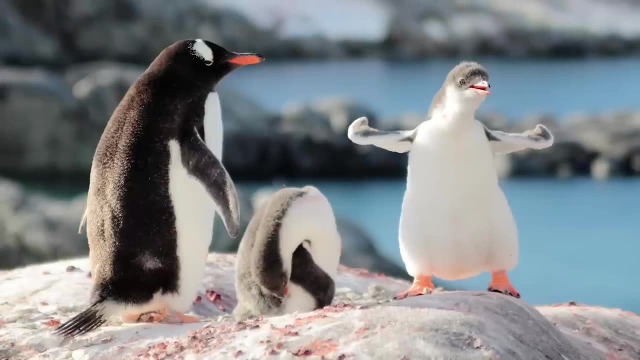 conditions, this realm is quite appealing. Penguins are the best example of animals who make the most of the Antarctic. Species include the emperor penguin, who can weigh almost 100 pounds, chinstrap penguins, who are named so for the black line across their chin, and gentoo penguins. 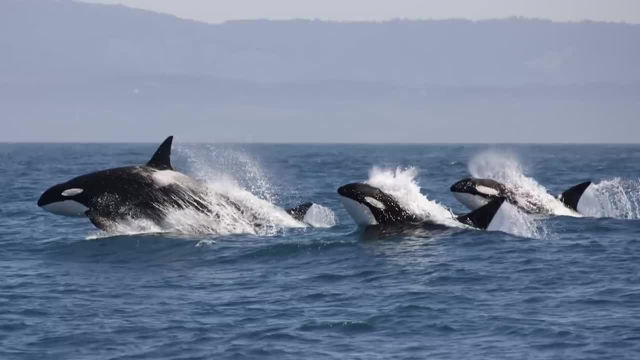 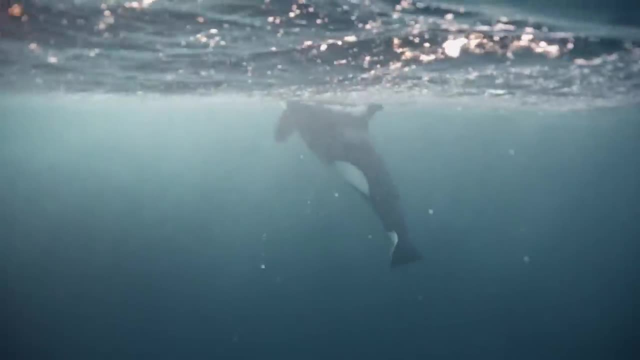 who evidently love it here. Patrolling the ice-cold waters of the Antarctic are pods of orca who, amongst other things, hunt penguins, seals, fish and squid. Other whales include humpbacks who, being filter feeders, feast upon large schools of Antarctic krill. 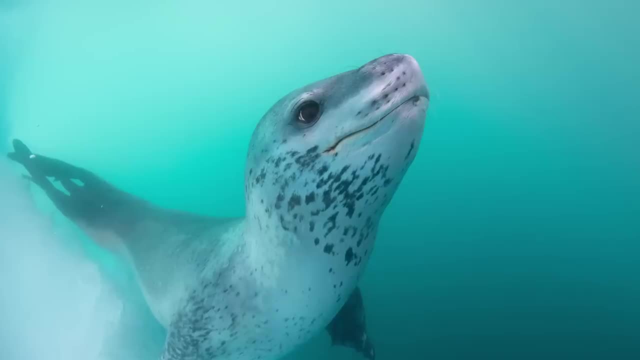 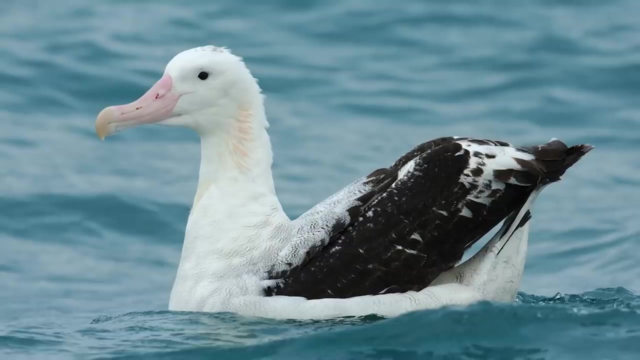 which measure no more than two and a half inches in length. Another aquatic threat to the penguins are leopard seals, who can also be found on the pack ice hiding from orcas. Seabirds include the wandering albatross, whose range extends to the southern regions of Australasia, Africa and the 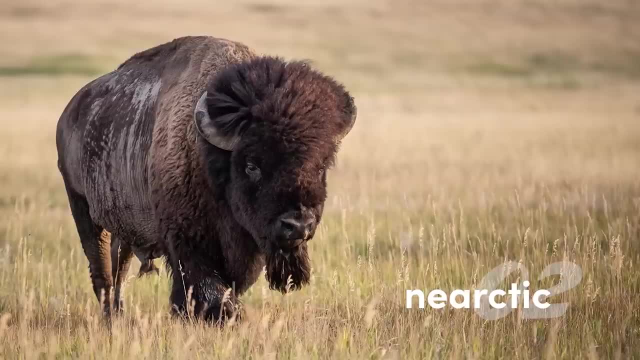 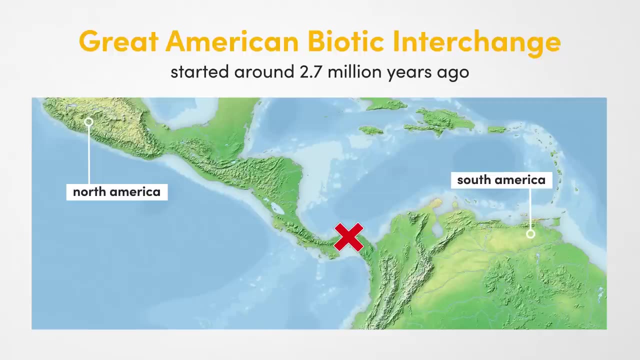 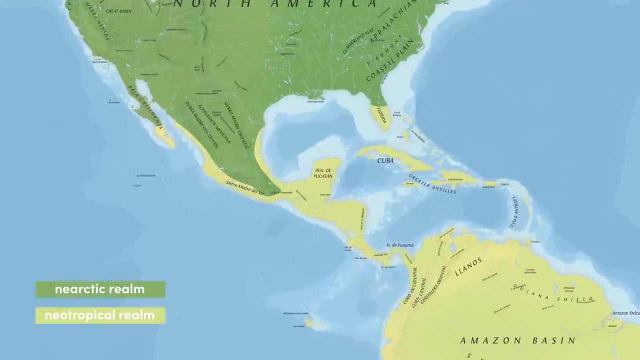 Americas. Up until 2-3 million years ago, North and South America were separated and the wildlife on each of these landmasses evolved independently. Today, these continents are joined by the isthmus of Panama, and the border of these realms corresponds almost entirely to the Arctic. 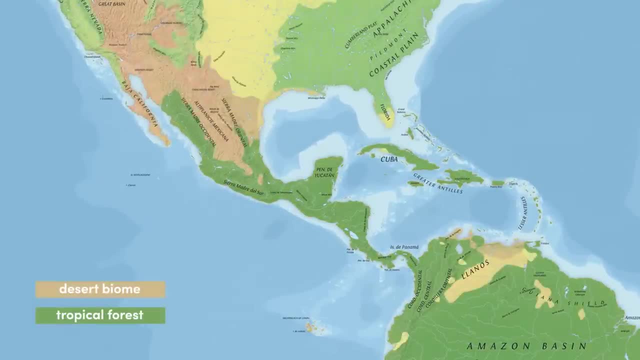 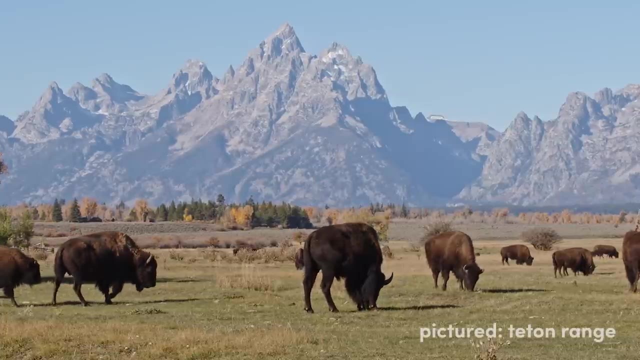 The Arctic is almost exactly with the junction of tropical forest and desert in the center of Mexico and a small region in southern Florida. The topography of the Nearctic is epic: It features the northern or western half of the American Cordillera, a chain of mountain ranges. 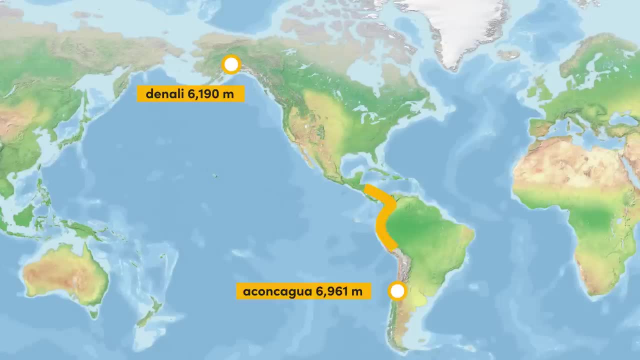 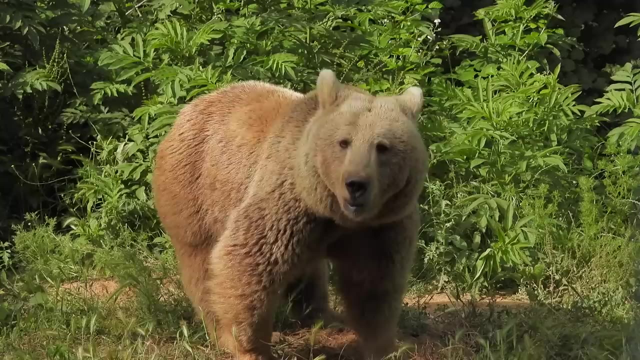 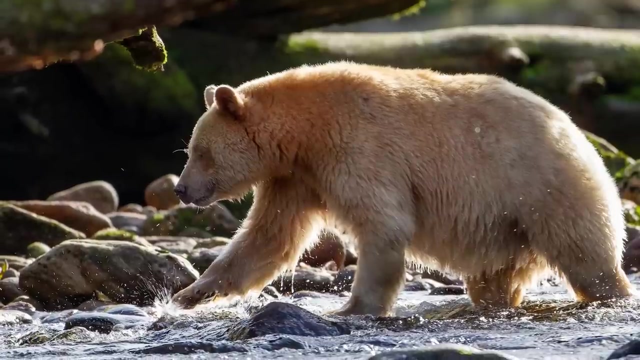 that stretches from Alaska to the southern tip of South America and is the defining geographical feature of the west coast. If there is one animal that North America is famous for, it's bears. Individuals range from the gigantic Kodiak bears in Alaska and rare magical spirit bears in British Columbia to the polar bears of the 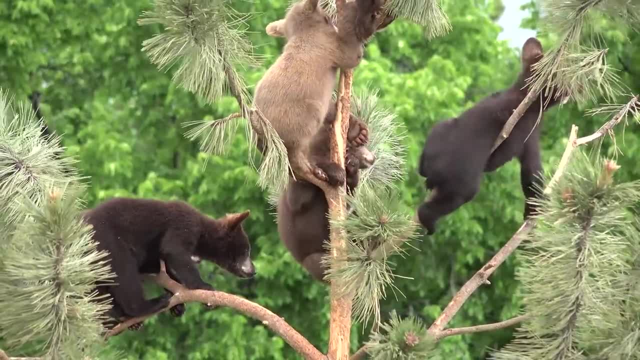 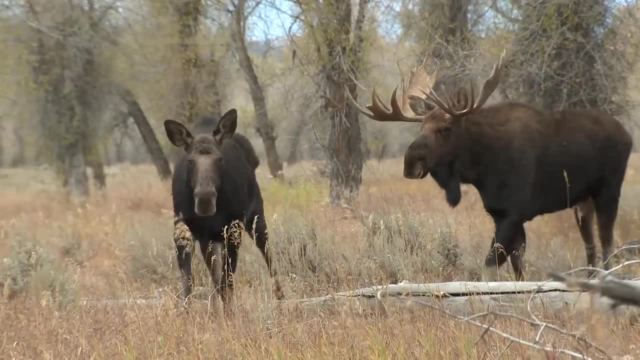 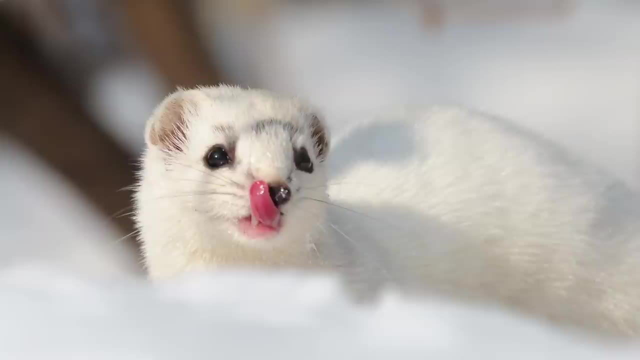 tundra and black bears, whose range extends to every corner of this realm. Moose traverse the boreal forests of the north, picking off bark leaves and twigs from willow, aspen and balsam fir trees. The world's smallest carnivore, the least weasel, is found in more open habitats. 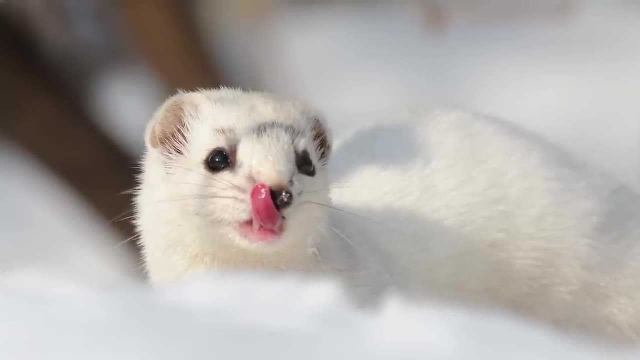 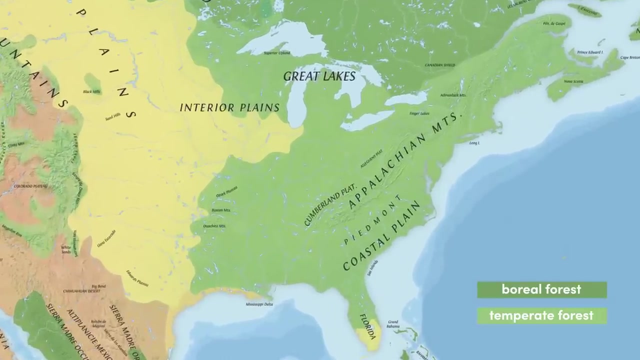 where it preys upon mice-like rodents, such as mice From Canada's tiger in the north to temperate areas further south. the eastern half of this realm is covered almost entirely in vast swaths of forest. The Nearctic's most iconic river is unquestionably the Mississippi the fourth. 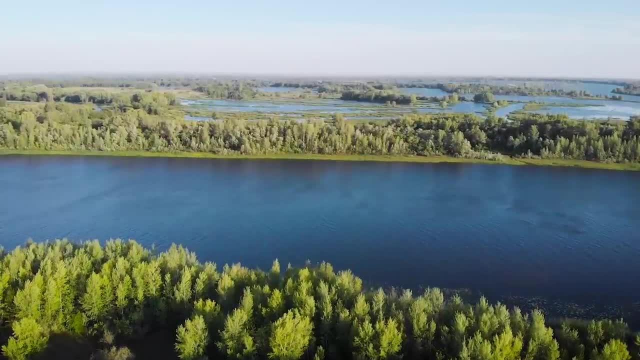 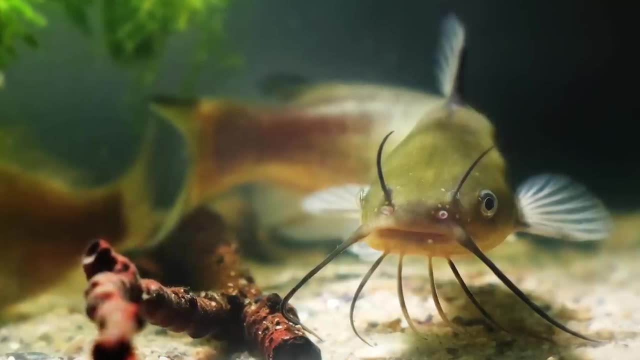 longest in the world and the fifth largest in terms of drainage area. The channel catfish, the most common catfish in North America, navigate the waters of the Mississippi with paddlefish, who are referred to as primitive for their lack of morphological advancements over the years. 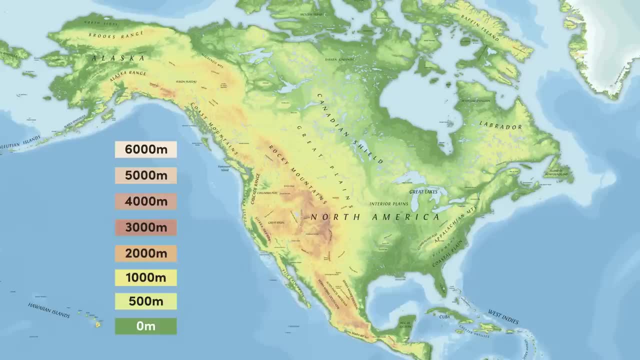 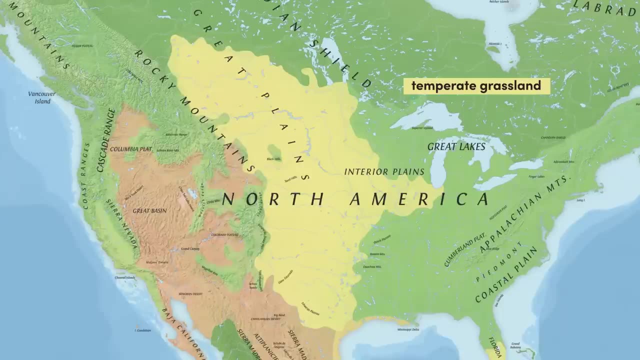 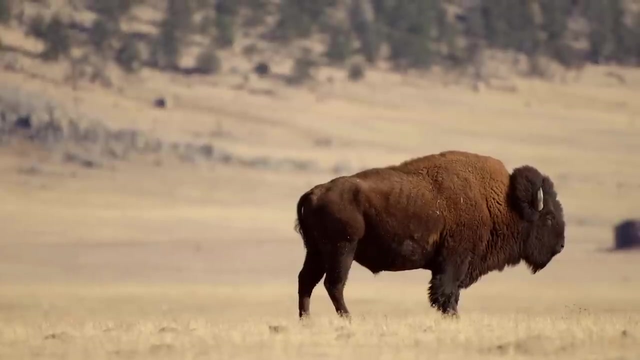 by their elongated, paddle-shaped rostrum. In the heart of the Nearctic, just east of the Cordillera, lies a large area of temperate grassland known in North America as the prairies. Here herds of pronghorn graze alongside American bison, the largest mammal in North America. 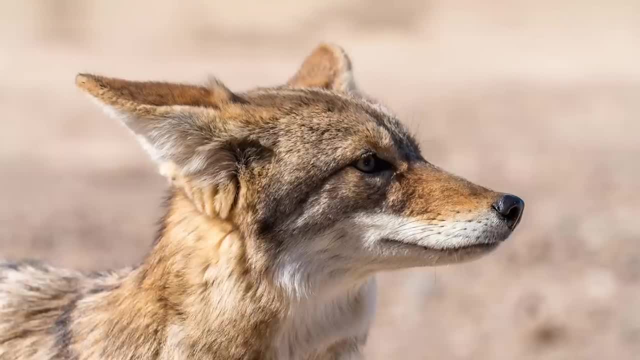 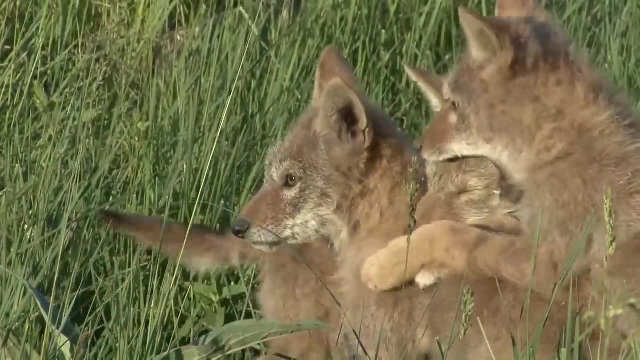 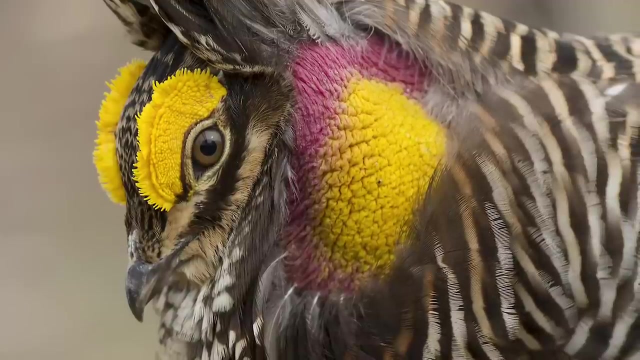 weighing almost 2,000 pounds. Interestingly, coyotes, who are also found here, were once named prairie wolves, but are no longer referred to by this name. One of the unique birds of the prairie is the greater prairie chicken. Males have bright yellow eyebrows and 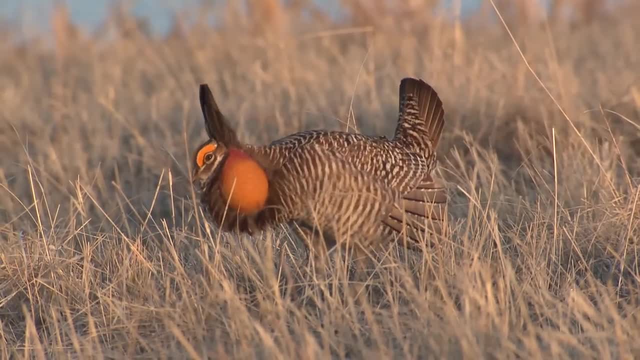 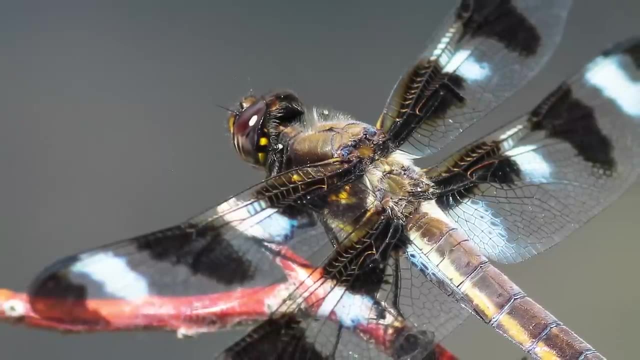 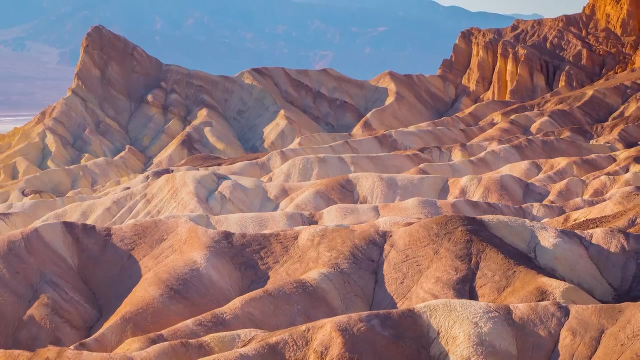 air sacs on their neck, the latter of which are used to make deep mating calls during breeding season. Insects include the 12-spotted skimmer, a colorful species of dragonfly, and the rusty patched bumblebee, who are vital for pollination but are currently endangered. The hottest place. 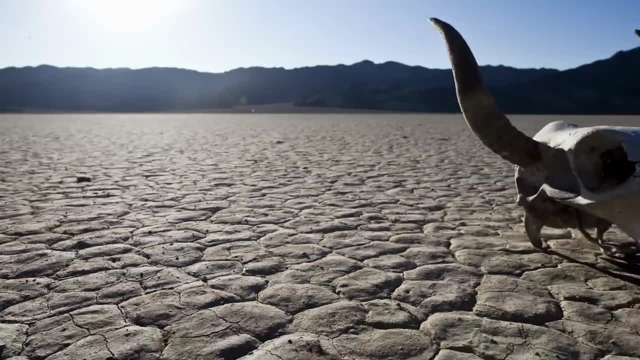 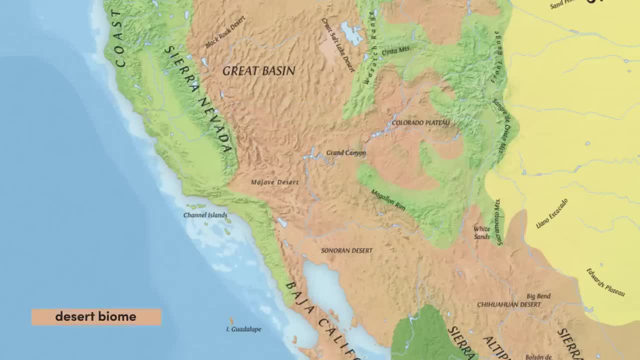 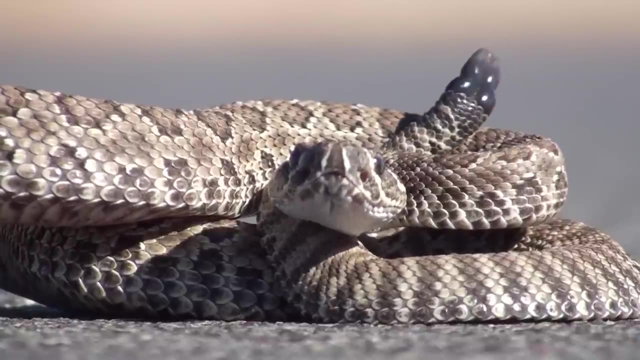 on earth is debated, but one location that shows up in every list is California's Death Valley. It is located in the Mojave Desert, which is part of a chain of arid areas stretching from the northern contiguous United States to central Mexico. If there is one type of animal, that 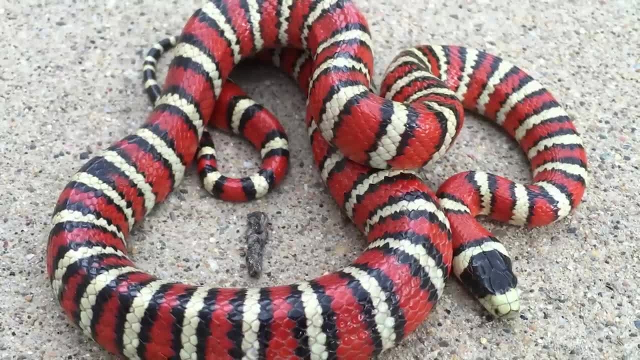 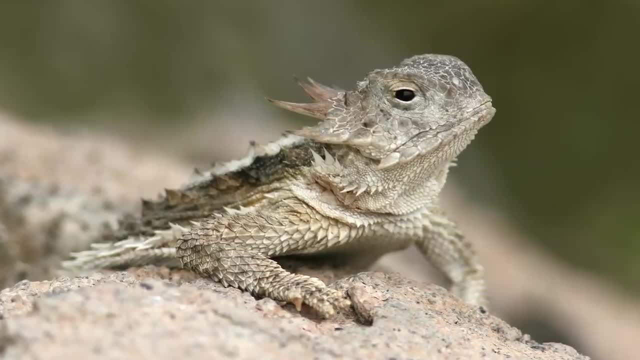 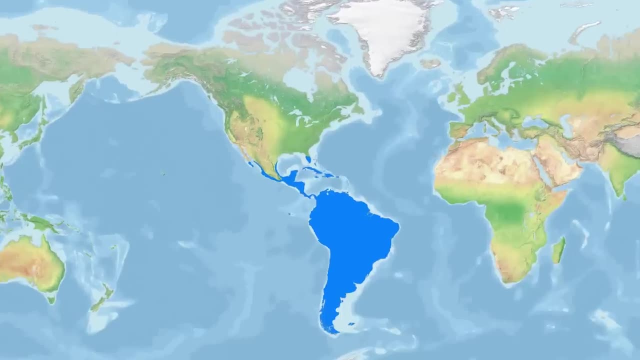 does well. here it's reptiles. Sonoran mountain kingsnakes and western rattlesnakes soak up the sun next to great basin collared lizards and prehistoric-looking desert horned lizards. The Neotropical realm contains six of the world's 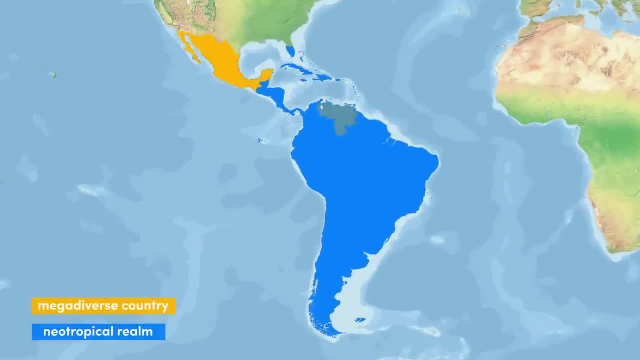 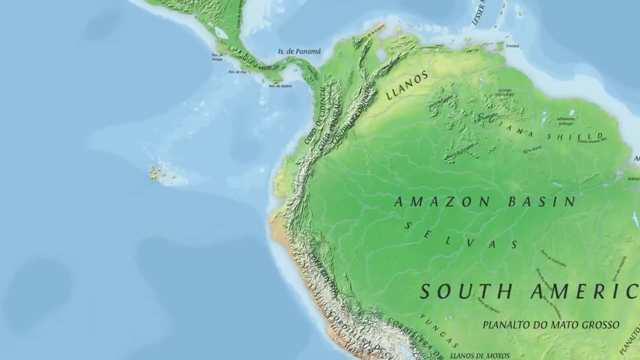 mega-diverse countries- Mexico, Venezuela, Colombia, Ecuador, Peru and Brazil, which is more than any other realm. Also included in the Neotropics is a chain of idyllic islands known as the Caribbean. The topography here is similar to the Neoptic, with a long stretch of mountainous. terrain, traversing the west coast, culminating in the highest peak in the Americas, Aconcagua, which stands at a staggering 6,900 meters. The lifeblood of this realm is arguably the greatest river on earth: the Amazon It is. 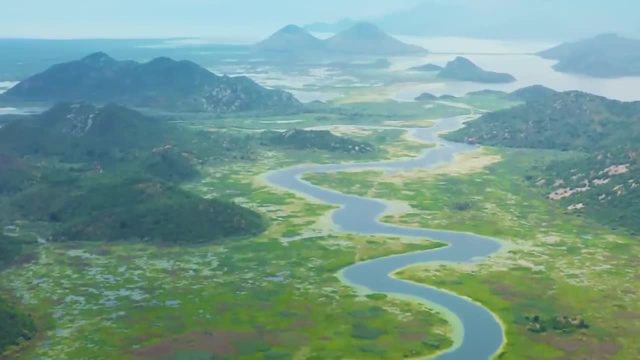 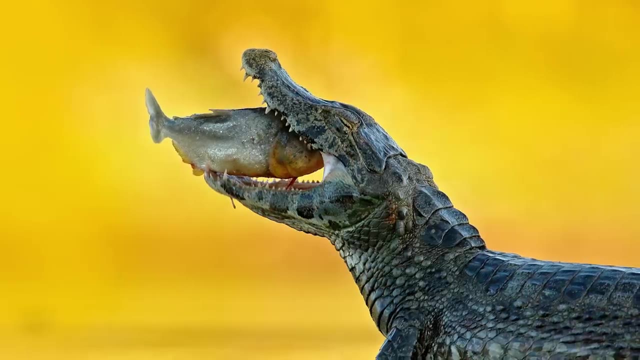 second only to the Nile in length, but at almost twice the size of the Congo, it is by far the largest in terms of drainage area, which sits in five of the six mega diverse countries. In these murky waters, shoals of red-bellied piranhas swim beside caiman. 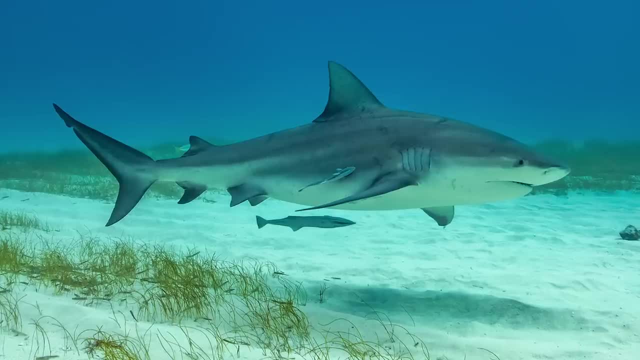 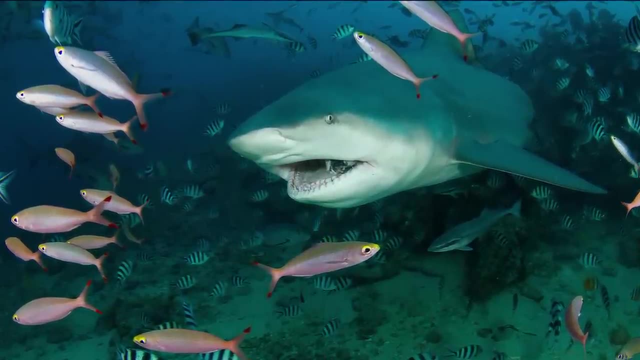 one of the largest reptiles on the planet and, perhaps most terrifyingly, bull sharks, which, like many other saltwater species, have been found 4,000 kilometers up the Amazon. On the banks of this great river lie vast expanses of tropical forest that stretch to its northern. 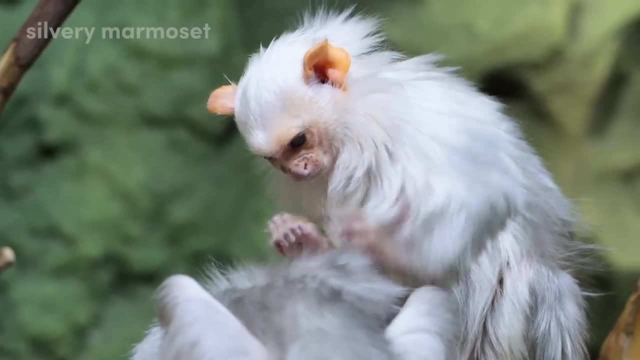 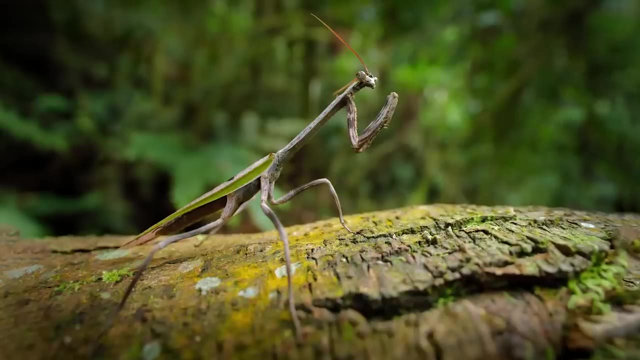 border with the Nearctic. The primates here are known as New World monkeys and include marmosets and howler monkeys, who can be heard communicating with each other in the canopy. The insects of this biome are plentiful and can be gigantic. The Hercules beetle is one of the largest in the world. 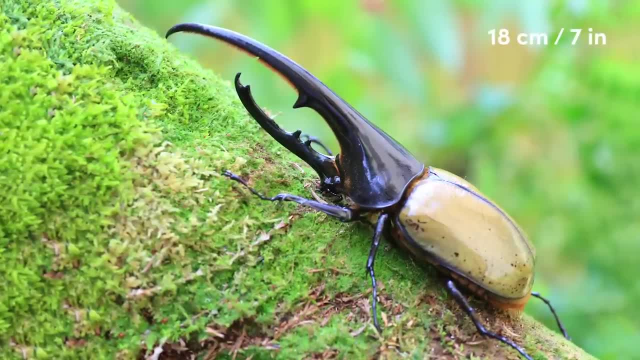 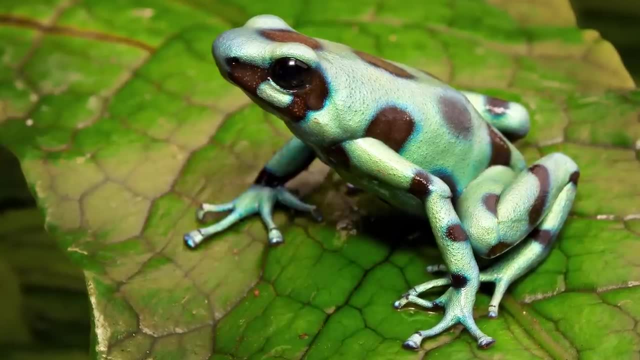 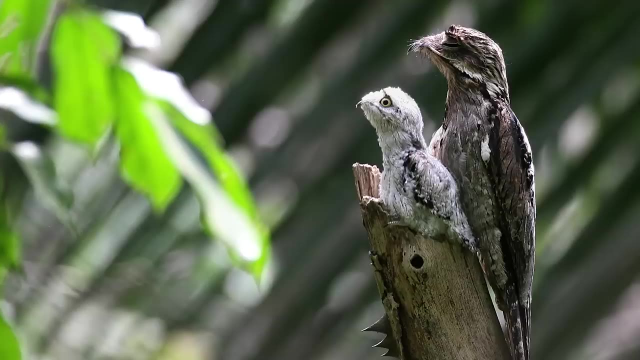 measuring up to 18 centimeters in length, including their horn. Poisoned dart frogs also abide here and display a range of vibrant colors from neon greens and blacks to fiery reds and oranges. Patoos are a wonderfully odd-looking bird family who, when their beady eyes are closed, 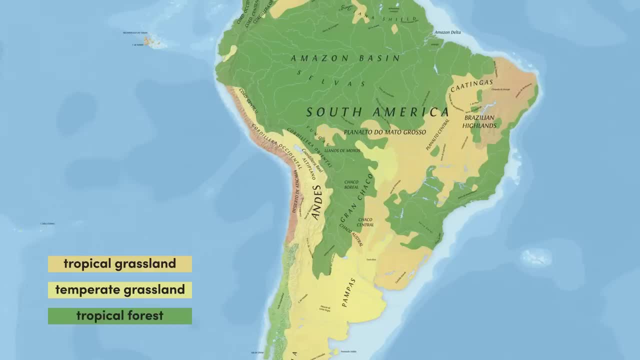 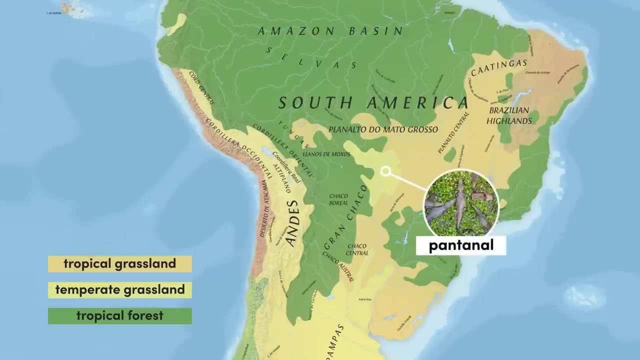 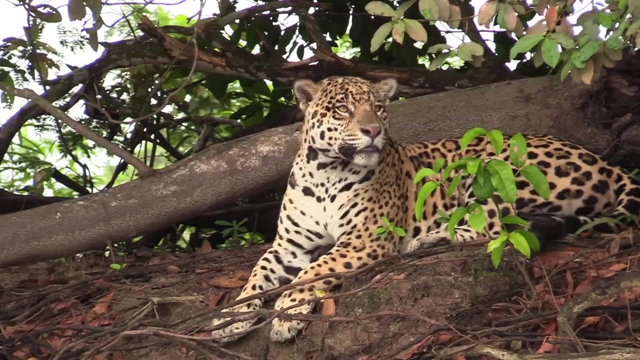 are incredibly well camouflaged for this habitat. Bordering the tropical forests are long stretches of tropical and temperate grassland. The Pantanal is a particularly interesting region. It is an area of flooded grassland known as the world's largest tropical wetland, home to the jaguar, the largest cat in the Americas. 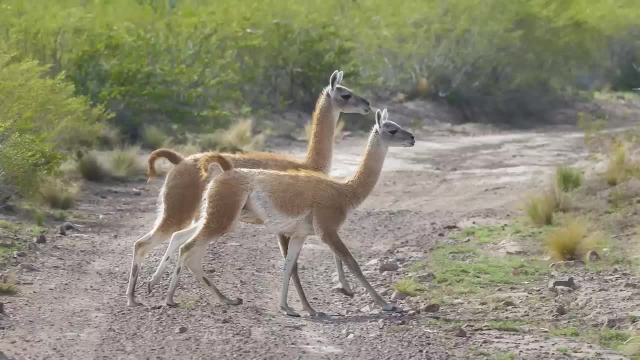 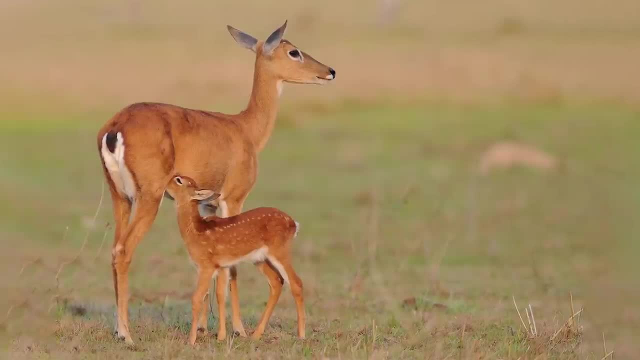 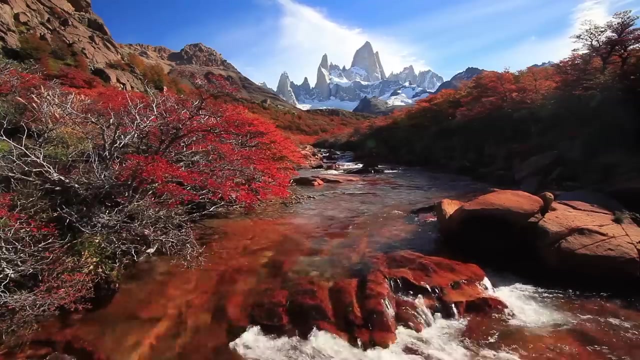 and the anaconda, the heaviest snake in the world. The pampas is a large area of temperate grassland found to the south. These fertile plains play host to species such as the pampas deer and the curious-looking pampas fox. Another stunning area that lies south of the pampas is Patagonia. 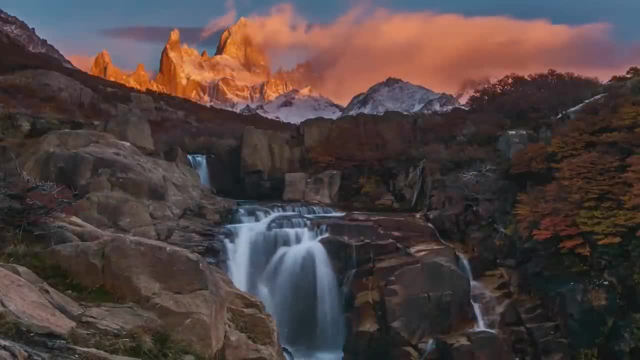 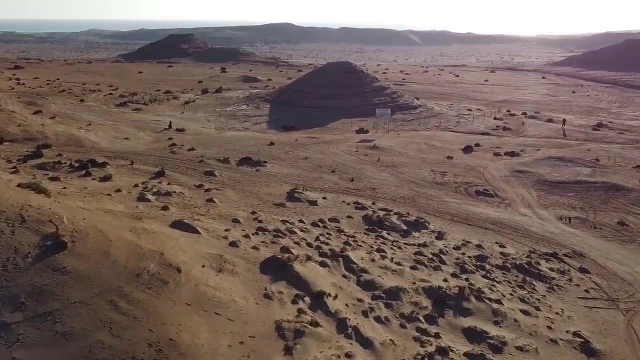 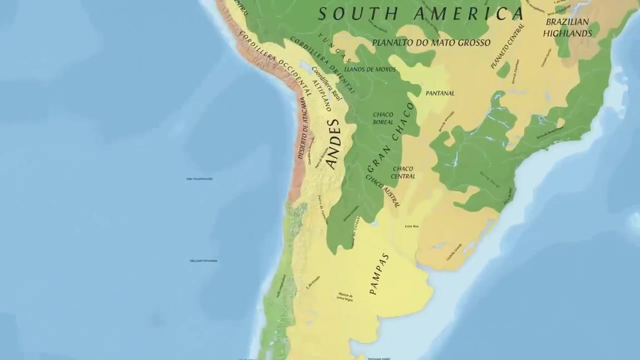 which terminates at the end of this realm, and is well known for its breathtaking landscapes. The last location that we'll discuss contrasts sharply with the wet, fertile areas previously discussed. The Atacama Desert sits on the western side of the Andes mountain range and is known as. 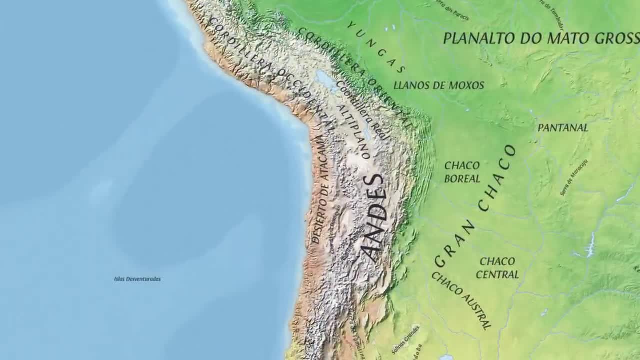 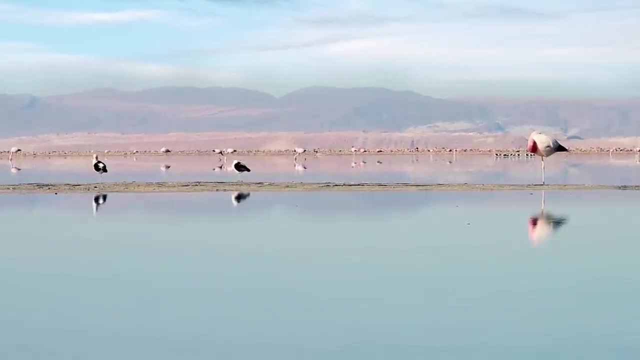 the oldest and driest non-polar desert in the world. due to the Andes blocking rainfall from the east, This desolate region is enjoyed by flocks of flamingos and is also home to the vicuña, a member of the camelidae family, who live at higher elevations. 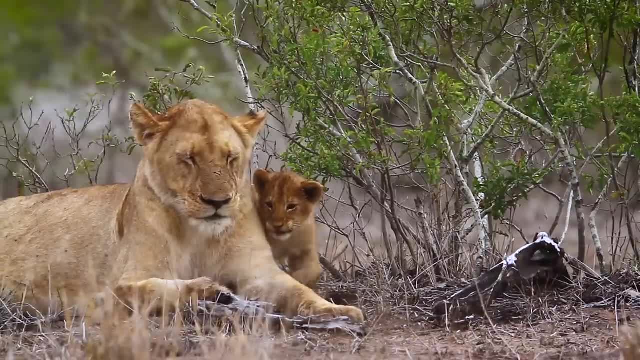 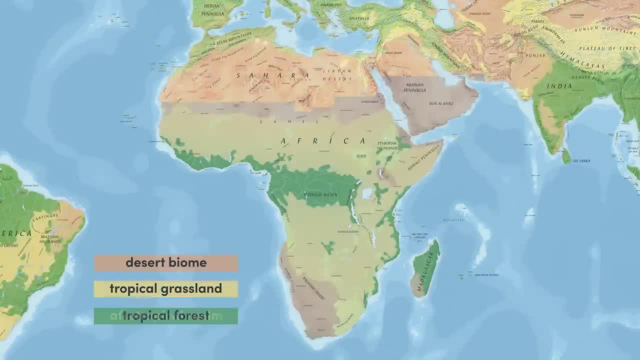 Unquestionably, the Afro-tropical realm is home to the most iconic wildlife on the planet. It makes up almost all of the African continent, and migration outside of this zone is near impossible due to a strip of barren land on its northern border known as the Sahara Desert. 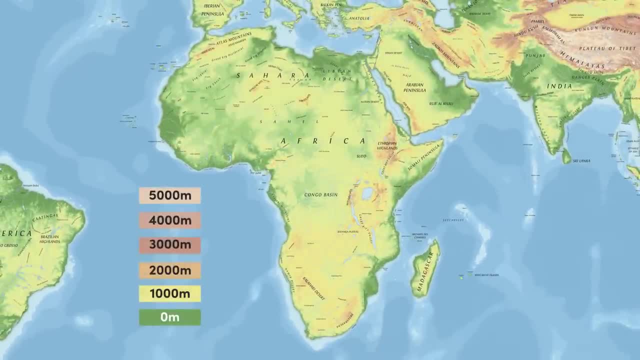 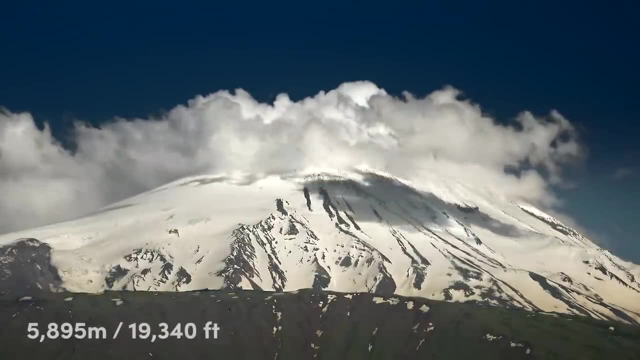 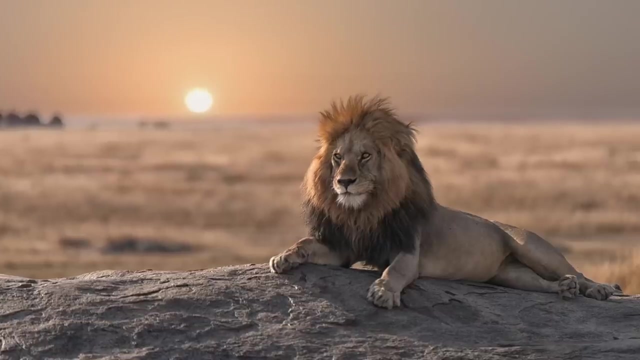 In comparison to other ecozones, the topography of this realm is one of its lesser-renowned features. although the volcanic Mount Kilimanjaro found in Tanzania ranks number four in the seven summits, surpassed by Denali by a mere 300 meters, The defining biome here is the savannah. 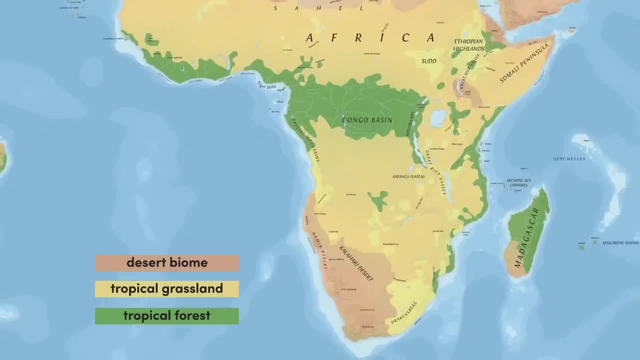 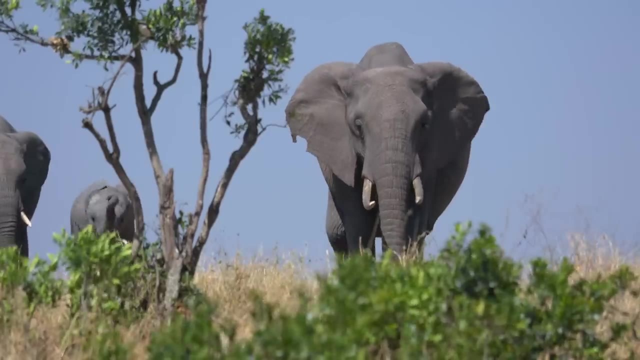 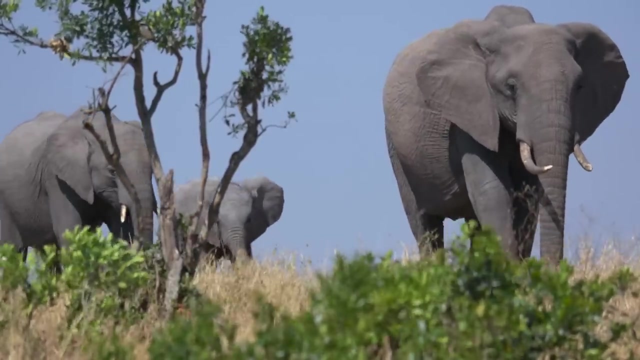 This vast region of tropical grassland stretches from the southern tip of the continent to the Sahara in the north and is broken up by patches of forest and desert. The animals of the savannah can be best described as gigantic. The largest terrestrial mammal is the African bush elephant. 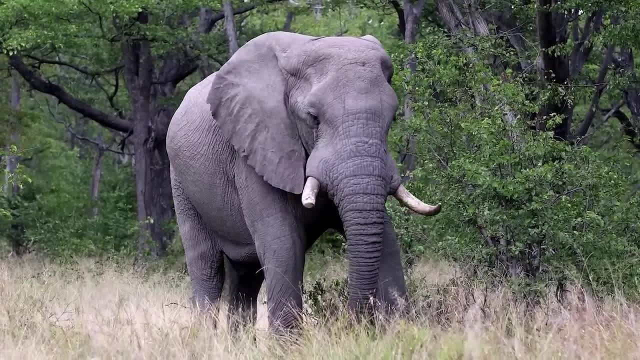 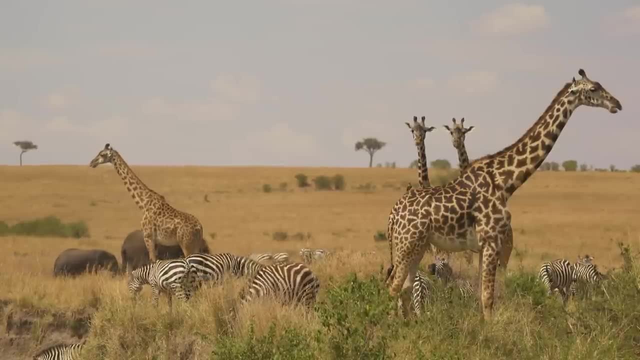 with the heaviest individual ever recorded in Angola, weighing a staggering 24,000 pounds. The fact that these herbivores have evolved to become so large is unsurprising, given the predators that roam these grasslands. Prides of lions can contain up to 40 individuals weighing 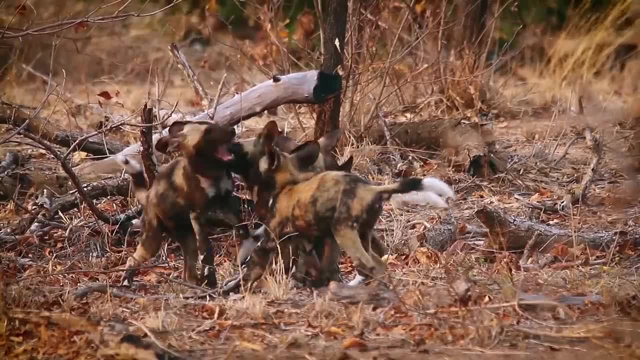 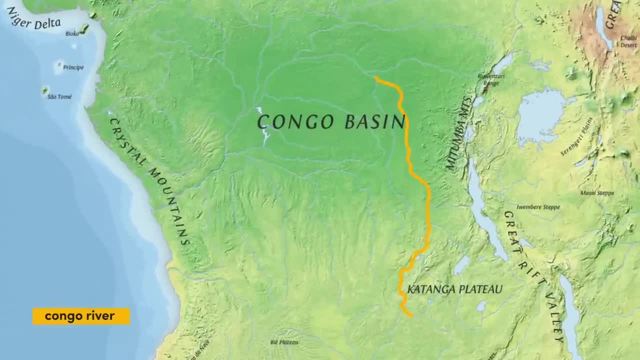 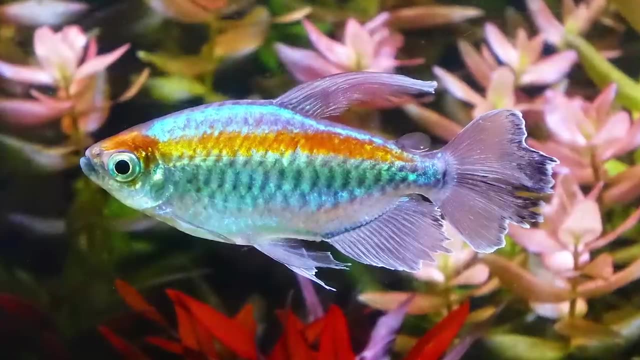 as much as 600 pounds a piece, and packs of African wild dogs can also reach 40 in number. At the heart of the Afro-tropical realm lies the Congo River, which, in terms of drainage area and average discharge, is second only to the Amazon. The Congo features many colorful fish, including the 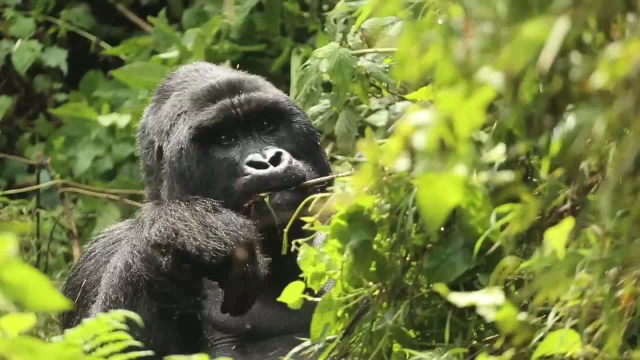 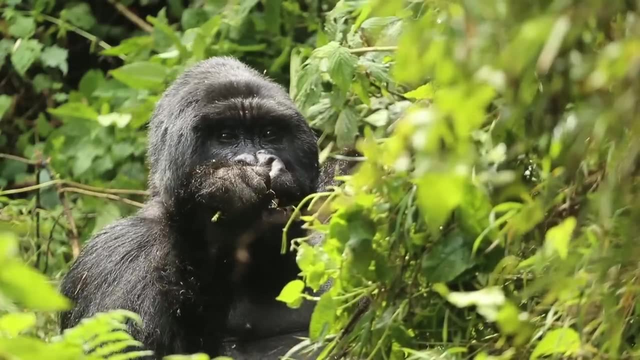 mullet and various species of freshwater pufferfish. Surrounding the river is a strip of tropical forest that sits directly on the equator and hosts the largest primates in the world. Eastern gorillas can weigh up to 440 pounds and unfortunately are critically endangered with less. 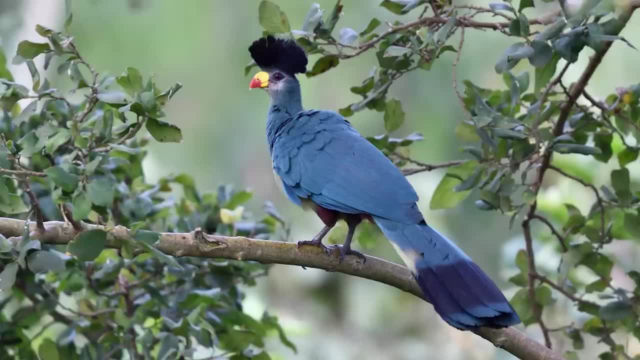 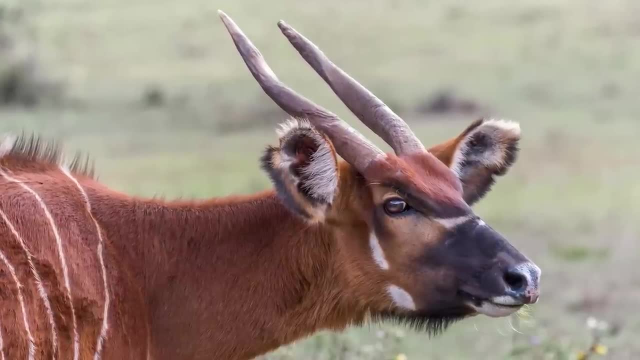 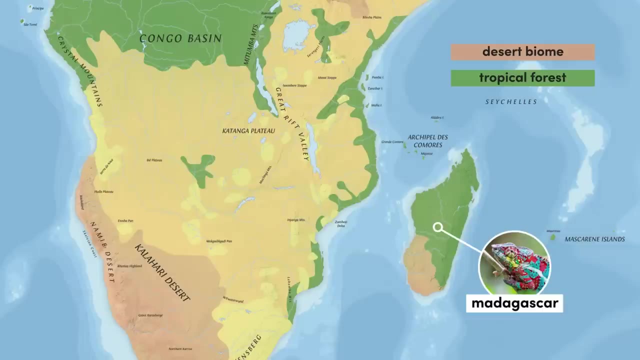 than 5,000 remaining in the wild. There are also many unique species, such as the great blue Turaco, the bongo with its beautiful horns and rich brown coat, and the red-legged running frog, which is also found on the savannah. The island of Madagascar is the fourth largest island in. 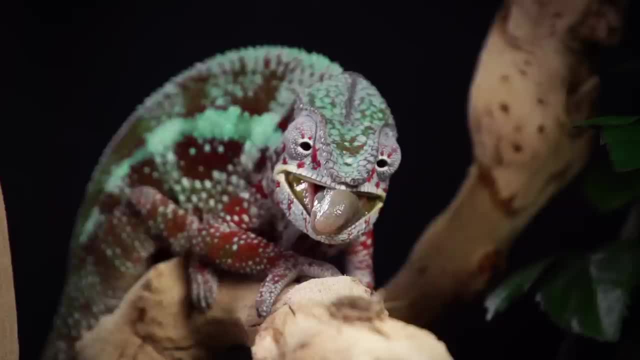 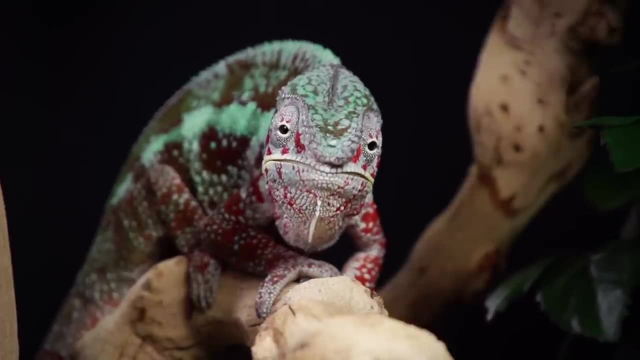 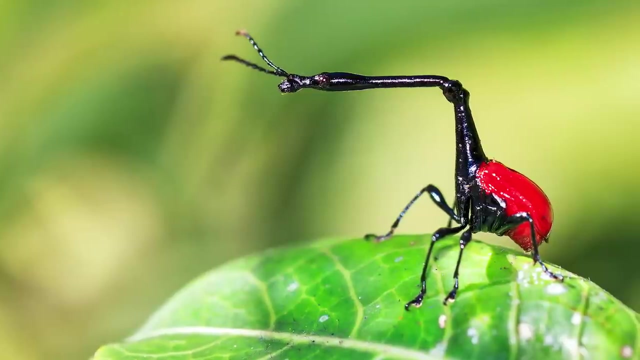 the world and one of the most biodiverse areas on the planet. Here, camouflage chameleons use their tongues as projectiles to snatch unsuspecting insects on whom they prey. The giraffe weevil is endemic to the island and is sexually dimorphic, with males exhibiting necks up to three times. 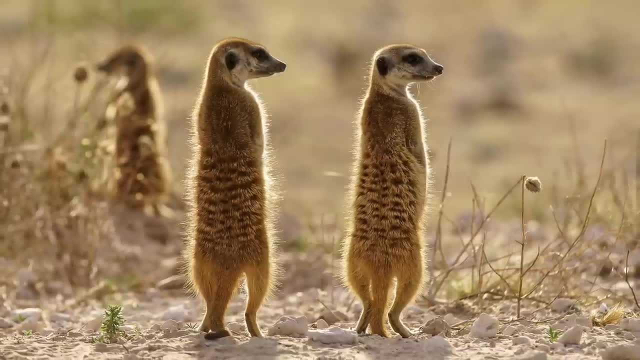 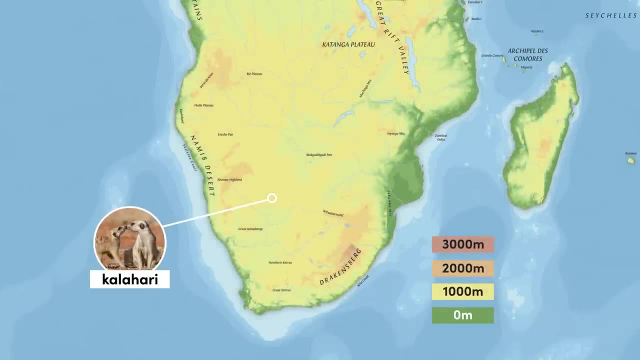 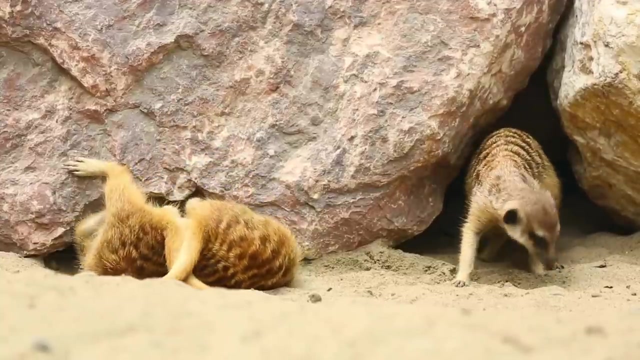 longer than that of a female. The last interesting feature we'll explore is the Kalahari Desert. This incredible stretch of land sits at 900 meters above sea level on the interior plateau of southern Africa. There are a surprising number of animals in this arid region, including meerkats. 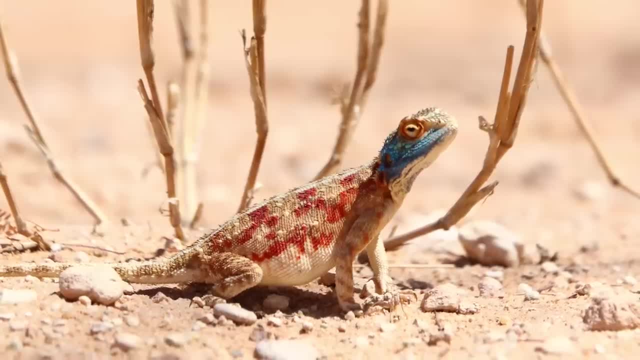 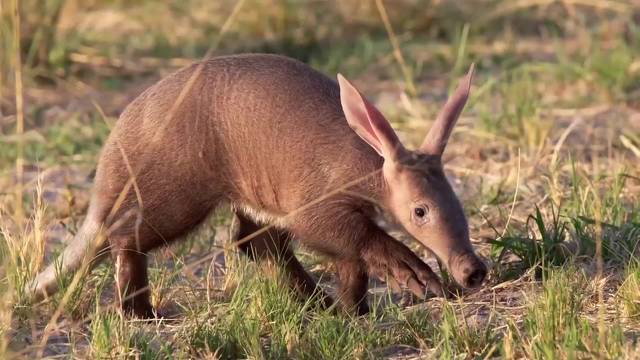 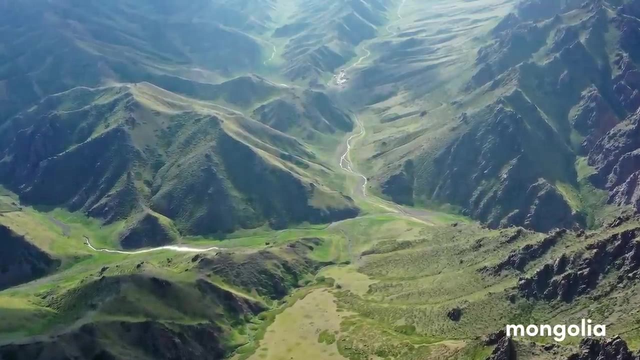 flocks of colorful flamingos, the blue-headed agama lizard and the aardvark, a largely nocturnal mammal whose range extends throughout most of sub-Saharan Africa. The Pale Arctic is the largest biogeographical realm, occupying 54 million square kilometers, which is well over twice the size of the. 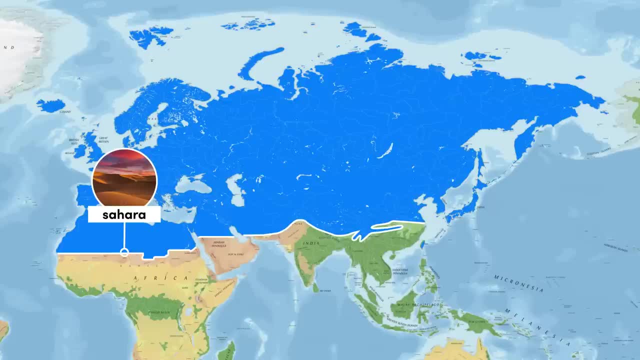 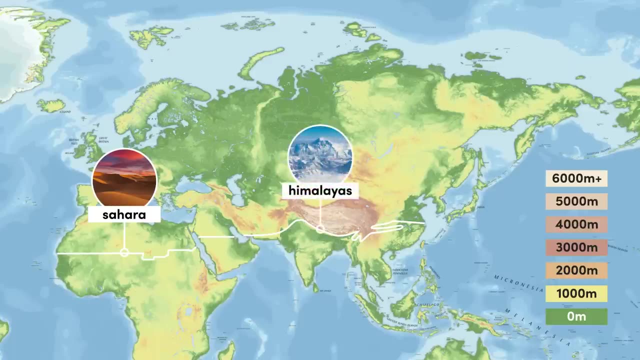 Nearctic, the second largest, In addition to the Sahara Desert, which sits on its southwestern border. this zone is separated from the Indo-Malayan realm by the highest mountain range on Earth, the Himalayas. There are several other mountain ranges that sit within this realm. 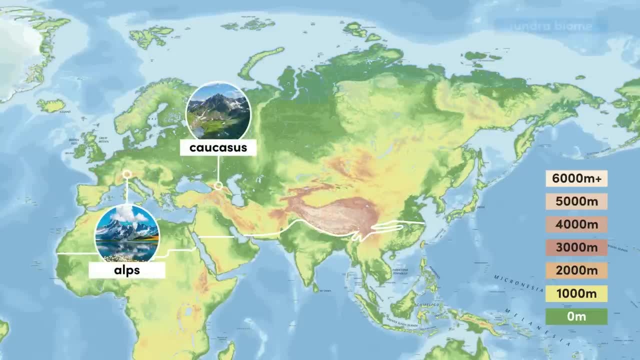 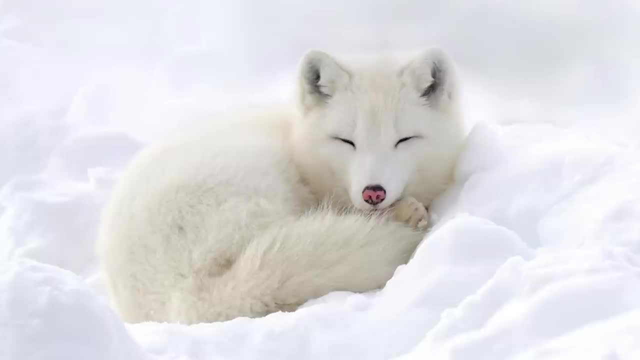 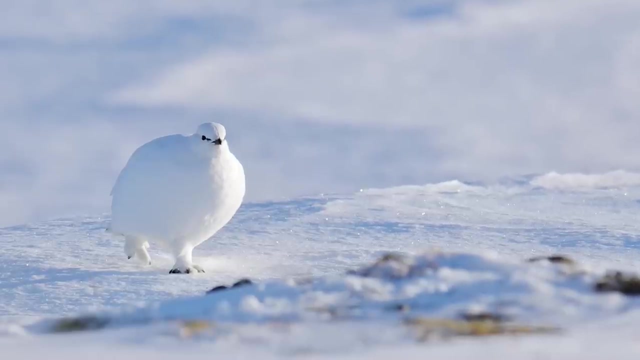 including the Caucasus and the Alps. At the top of the Pale Arctic lies the tundra. The animals here equipped for the freezing conditions, and many of them exhibit white camouflage, including arctic foxes and wolves, and birds such as rock ptarmigans and snow geese. beneath the tundra lies a strip of 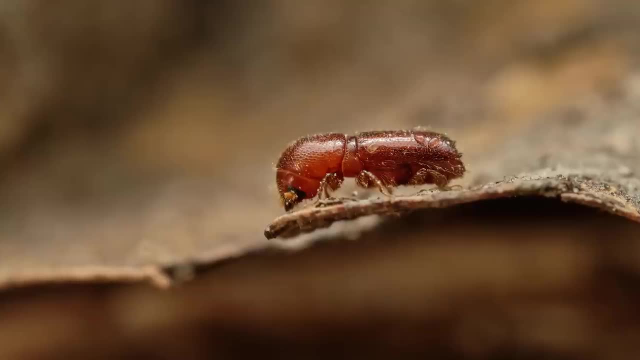 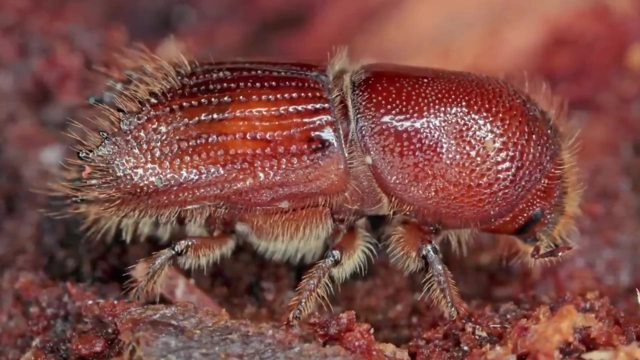 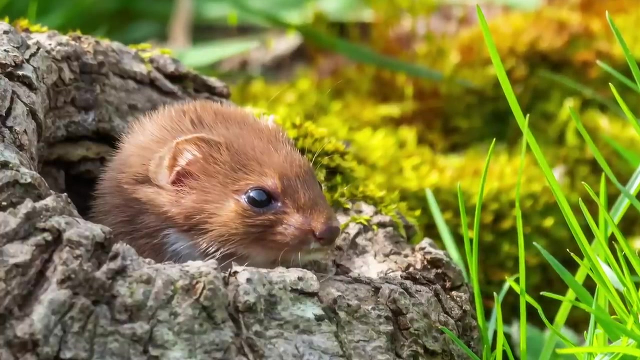 boreal forest, known as the tiger. many species of insect thrive in the boreal zone. the european spruce bark beetle is considered by some to be a keystone species and leaves a fascinating trail of destruction in the spruce it devours. one of the world's most intimidating creatures, abides. 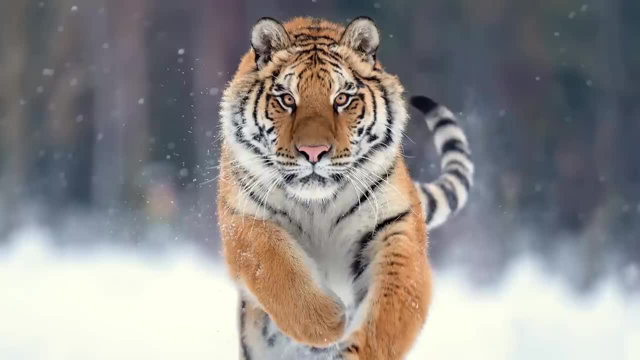 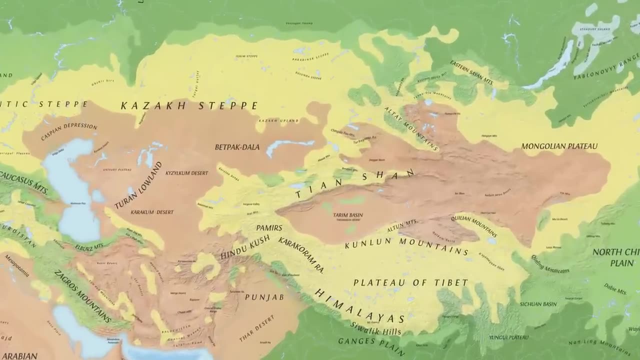 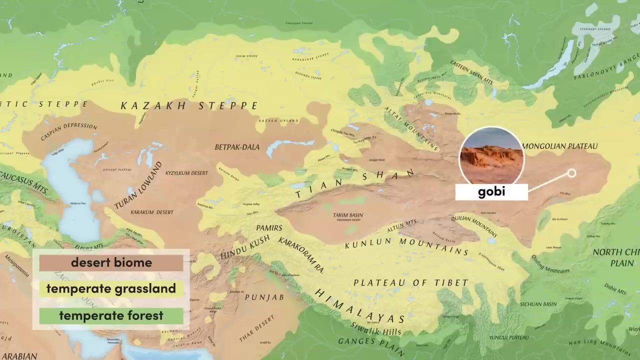 only in the boreal forests of far eastern russia the siberian tiger, the largest member of the philidae family. the area south of the boreal forest can be best described as a patchwork of temperate forest, temperate grassland and desert. the gobi desert sits northeast of the tibetan. 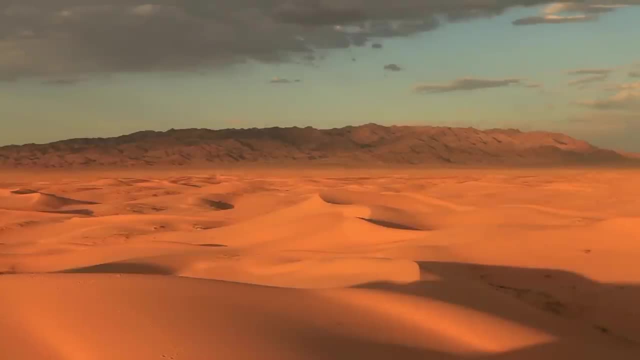 plateau and is one of the most inhospitable places on earth, with wind chill. temperatures can range from mild to high temperatures, and temperatures can range from high to low temperatures to high temperatures, and temperatures can range from minus 40 degrees centigrade in the winter. 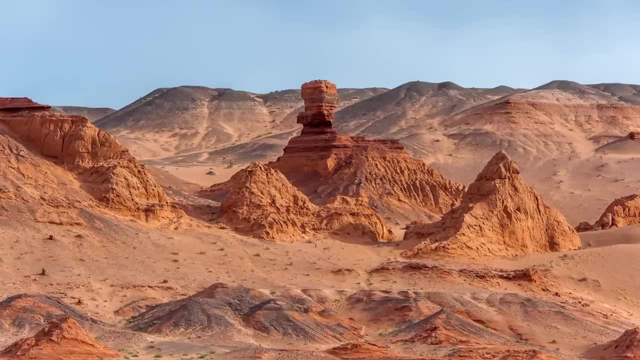 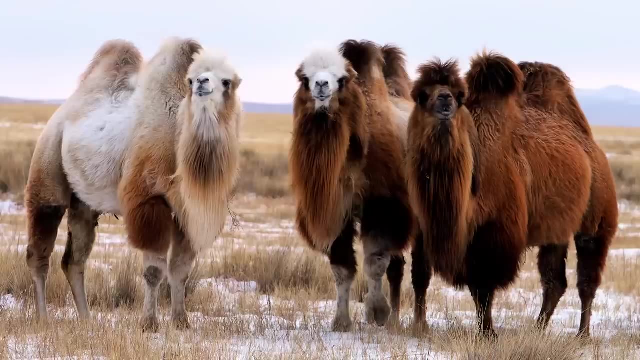 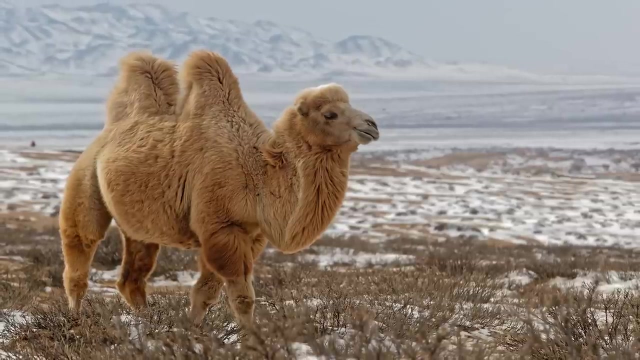 to positive 45 in the summer. although there are sand dunes here, most of the landscape is made up of flat, barren basins and colorful rock formations. one of the few mammals to excel in this habitat is the bactrian camel, which exhibits thick fur to stave off the frigid gobi knights. 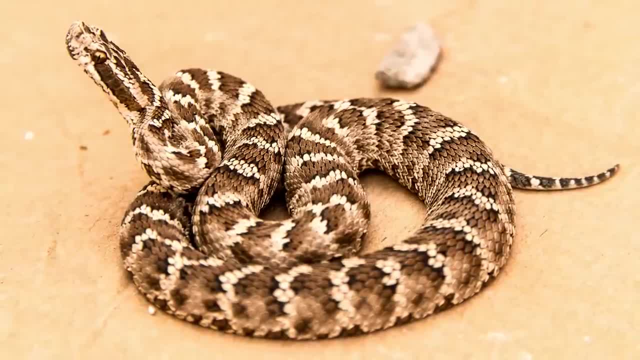 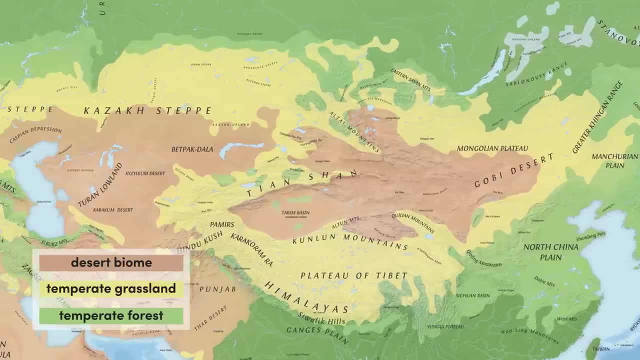 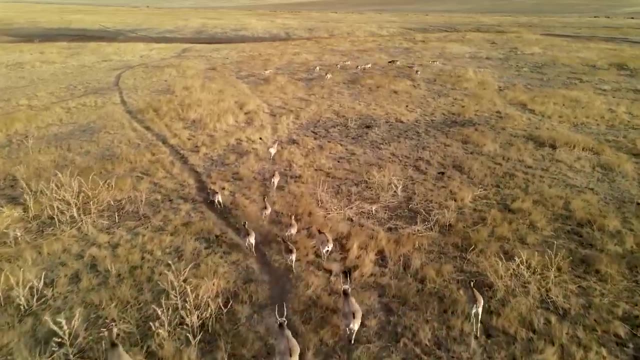 there are also several species of pit viper endemic to the gobi, including the hales or siberian pit viper. temperate grassland in the pale arctic is referred to as step and is generally found in the transitional zones between desert and forest, where environmental factors such as precipitation are enough to 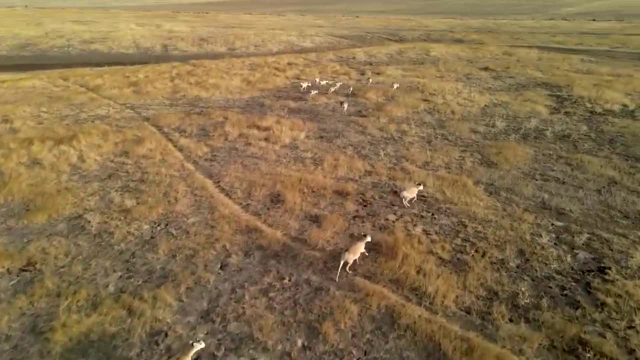 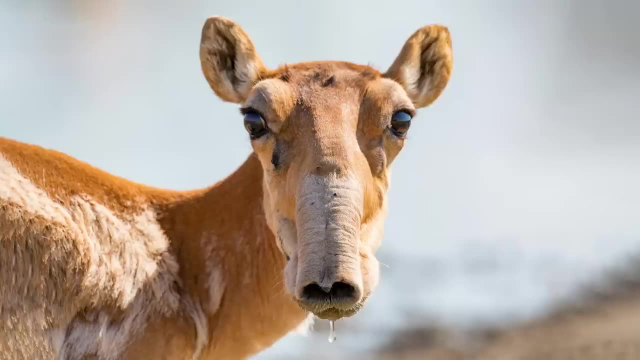 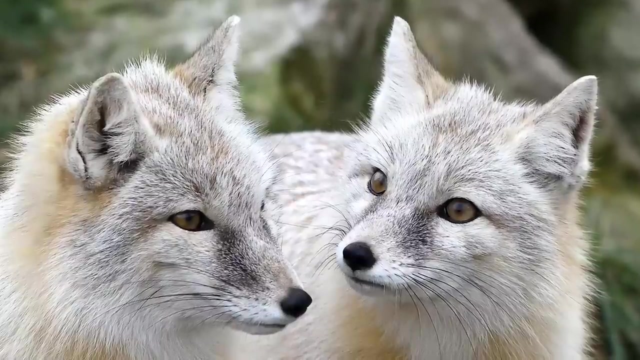 support the growth of grasses, but not sufficient for large amounts of trees. the volga river passes through the pontic step and is home to the colorful russian sturgeon on land. animals include the critically endangered saiga antelope, various species of fox and the majestic step eagle. 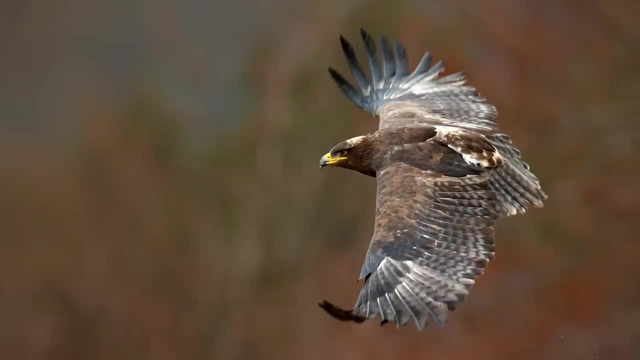 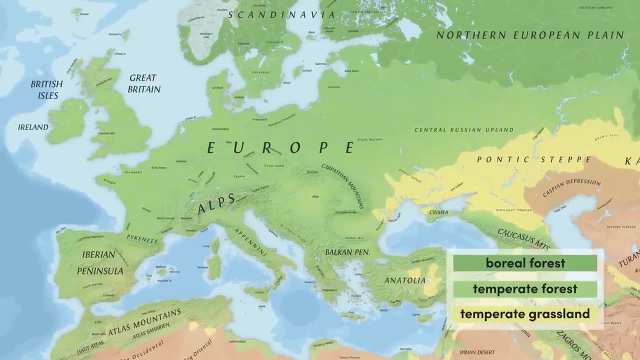 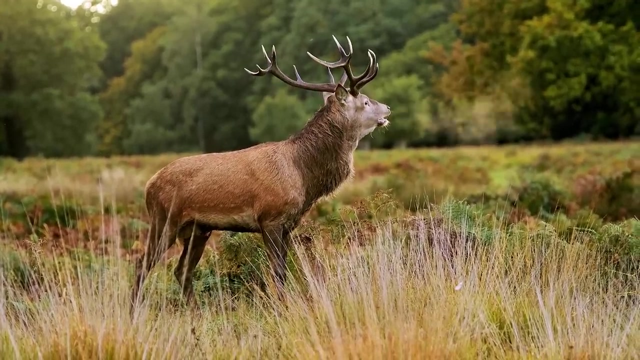 who would most likely have preyed upon the guinea pig, which is now extinct in the wild and is instead domesticated. the largest expanse of temperate forest is found to the west and makes up almost all of europe. deer are common here and will mill about peacefully beside pigeons whose appearance 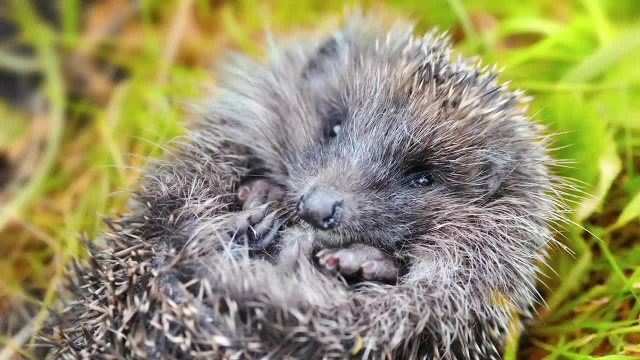 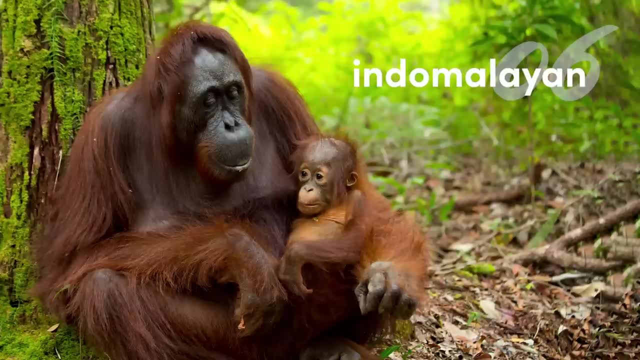 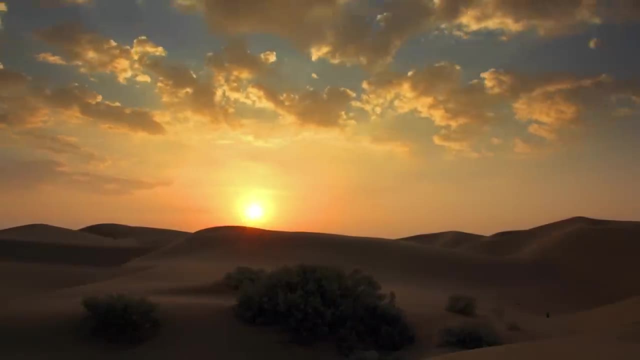 varies considerably between realms: the western european hedgehog and the european badger, the united kingdom's largest land predator. the indomalian realm sits to the south of the pale arctic, on the other side of the himalayas. its mainland body stretches from the thar desert in the west, which sits on the border of india, and 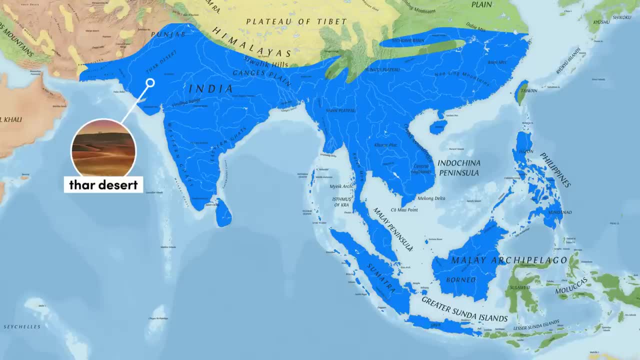 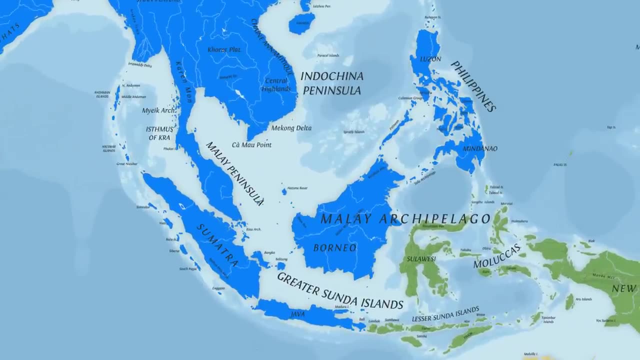 pakistan to southern china in the east. beneath are its island components, made up of the philippines and half of the indonesian and malay archipelagos, with the exception of the himalayas. its topography is relatively flat, especially in comparison with other zones and the 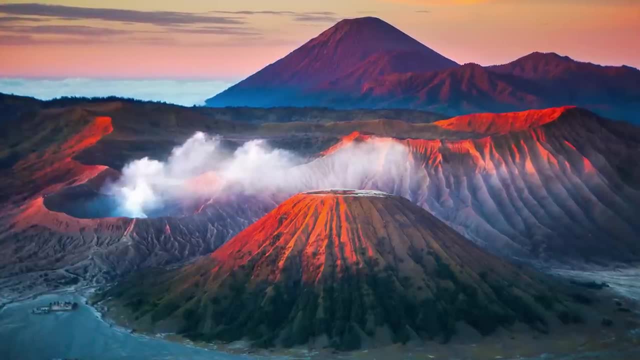 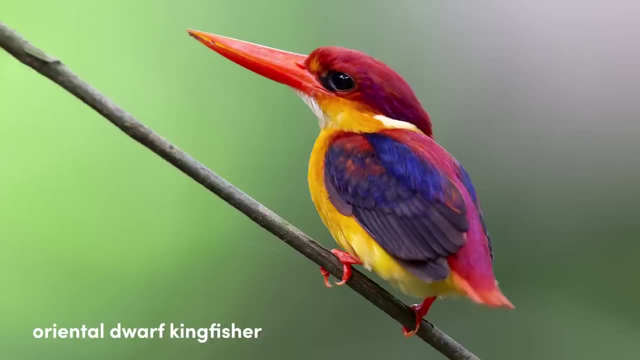 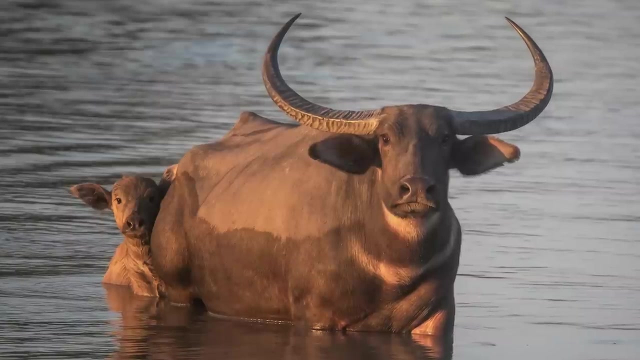 south of the philippines. although the islands of indonesia are a well-known volcanic hotspot, this realm is made up almost entirely of tropical forest, which, unsurprisingly, is home to an astounding amount of biodiversity, including the asiatic version of africa's big five. various species of water buffalo can be found in the tropical and subtropical forests of this. 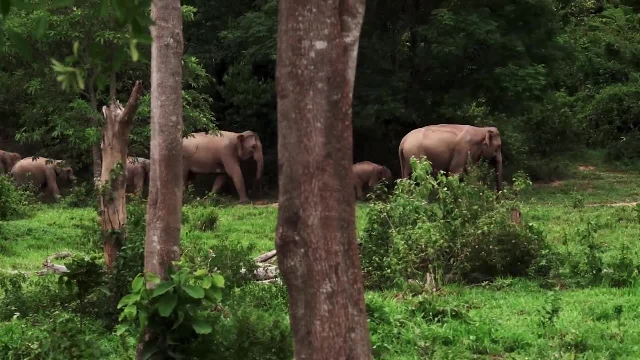 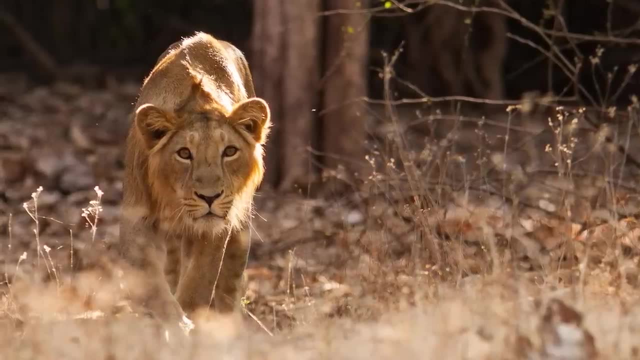 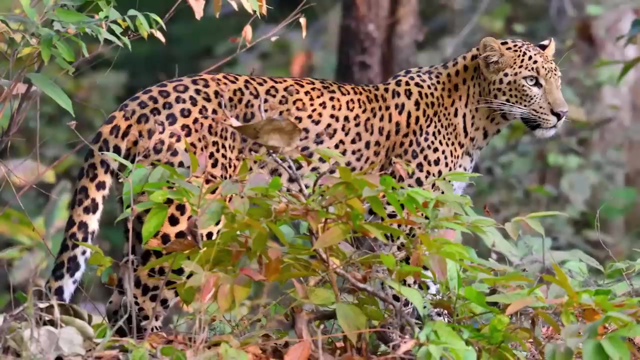 region. alongside asiatic elephants which, although smaller than their african counterparts, can still reach up to 13 000 pounds, large felines of this realm include the asiatic lion, an endangered but heavily protected subspecies of lion found only in india's gur forest, and the leopard, which, between its eight subspecies, has an 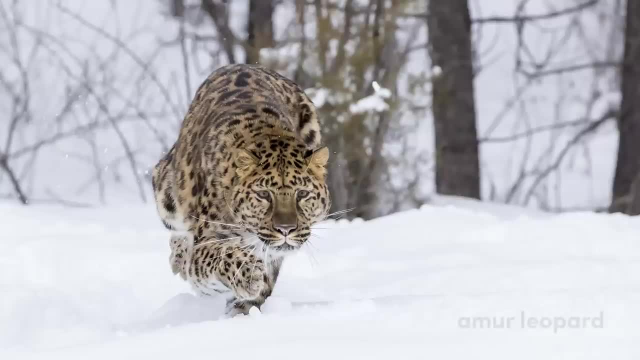 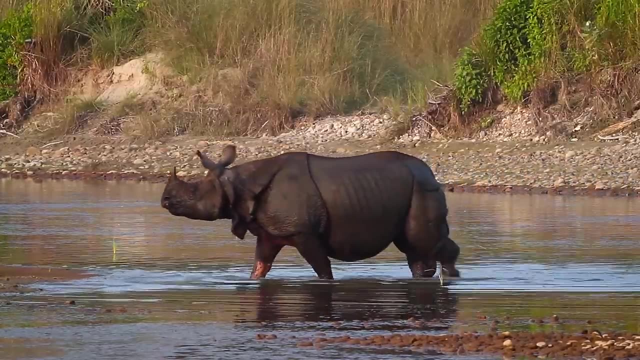 unusually large range from the southern tip of africa to far eastern asia. completing the big five are three species of rhinoceros, including the indian rhino, also known as the greater one-horned rhinoceros, whose numbers have risen from a bleak 600 in 1907 to 300 in the late 19th century. to the 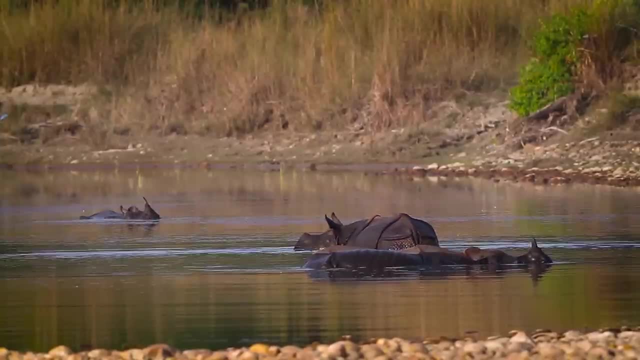 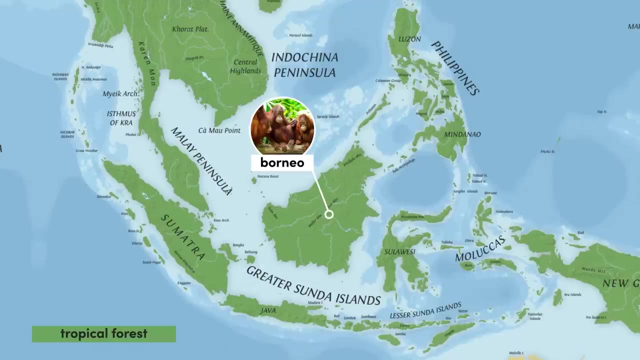 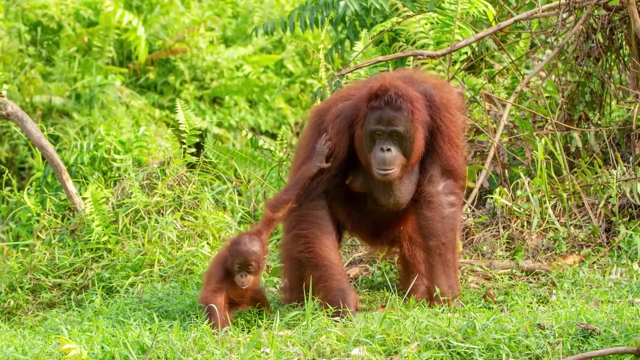 age of 75 to over 3 500 in mid 2015, thanks to valiant conservation efforts. another area renowned for its wildlife is the island of borneo. orangutans here will live for up to 50 years. they are mostly arboreal, and they're also found on the island of sumatra. 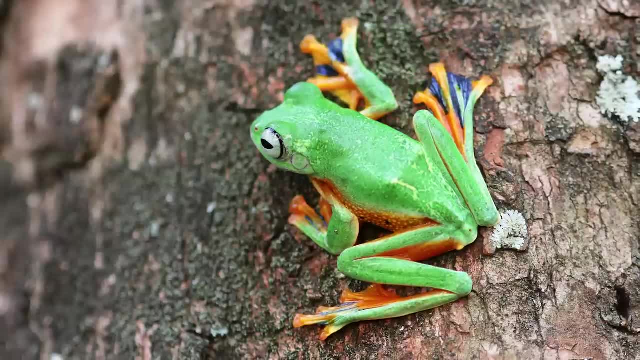 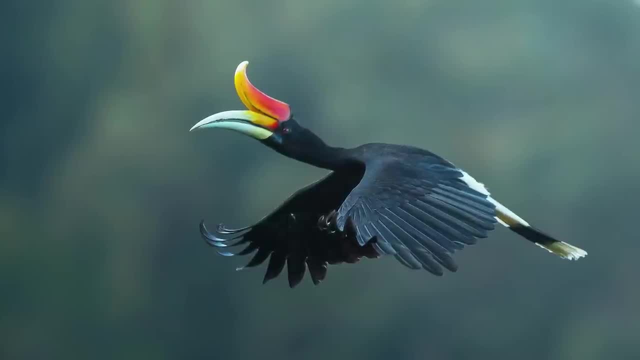 the wallace's flying frog is also arboreal and will use its webbed feet to glide from the treetops when threatened. one of the many colorful birds on the island, the rhinoceros hornbill, secretes a tinted oil from their preen gland when grooming, which is thought to give their 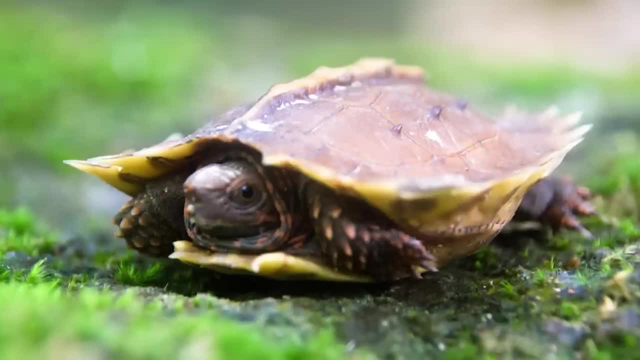 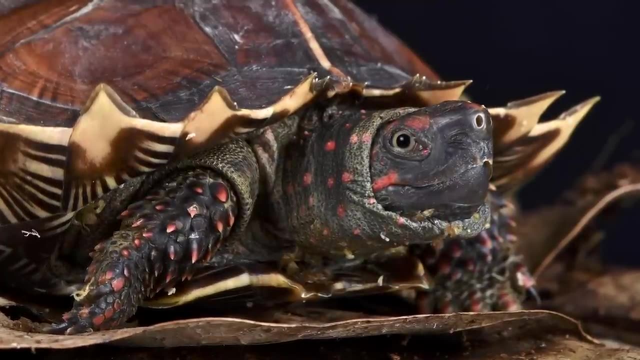 bill and cask its red tint. the spiny turtle is one of the most unique species of reptile and, although they are found throughout southeast asia, are classified as endangered, initially mapped by alfred russell wallace in the 19th century, the southeastern border of this realm. 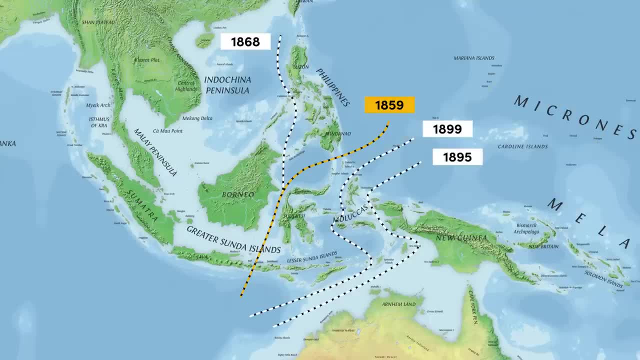 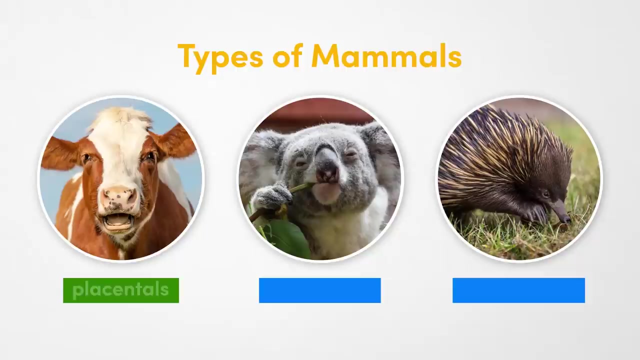 has been subject to much debate over the years, but lies somewhere between the islands of borneo and java and new guinea, on australia. this faunal boundary is known as the wallace line and, quite frankly, is fascinating for context. there are three living subgroups of mammals: placentals, marsupials and monotremes. 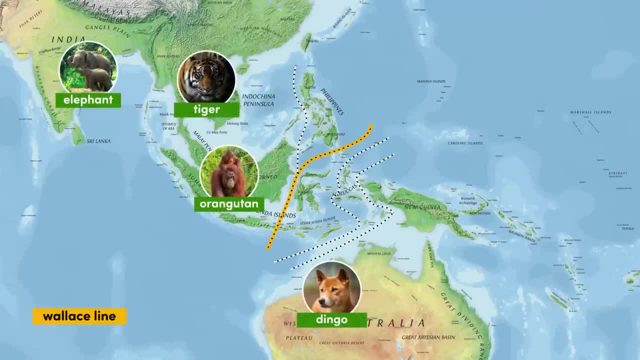 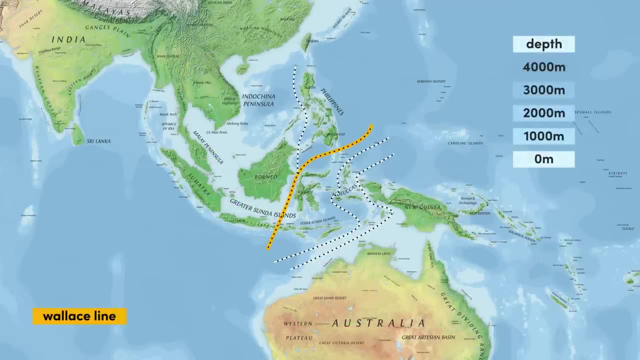 while there are some placental mammals in the australasian realm, there are no marsupials or monotremes east of the wallace line. it is thought that this separation is due both to continental drift and changing sea levels, with the wallace line representing a historically 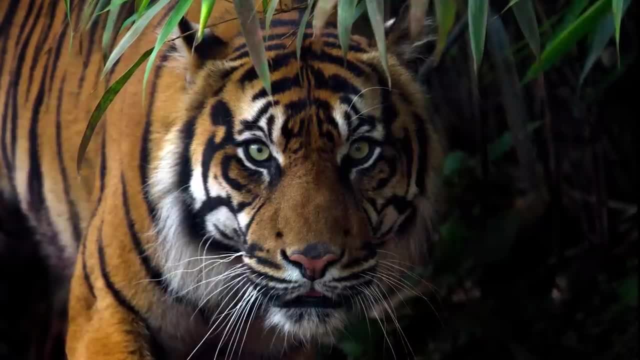 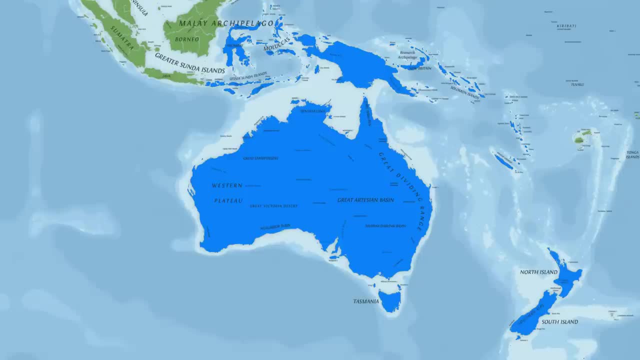 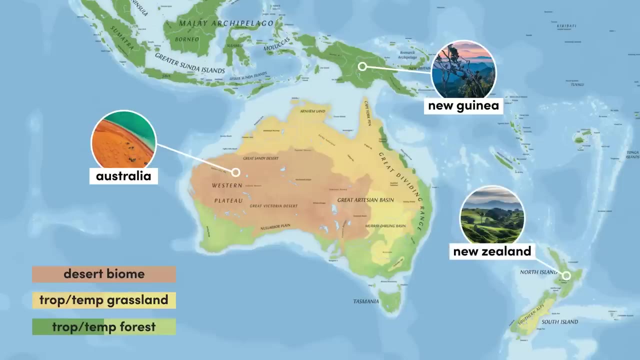 difficult boundary to cross for mammals who can't fly or be transported by humans. the australasian realm is positioned on the other side of the wallace line and comprises new guinea, australia, new zealand and several other smaller island nations. the highest peak in the region is found on new guinea and is over twice the height of. 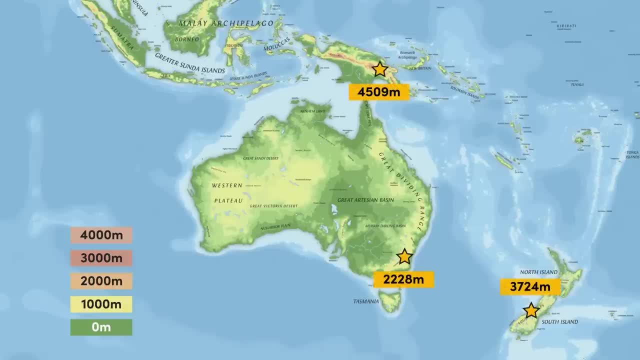 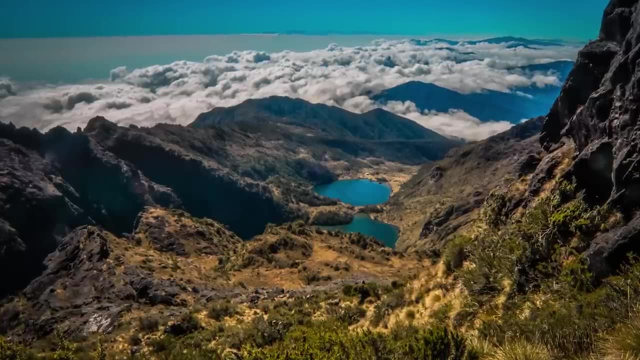 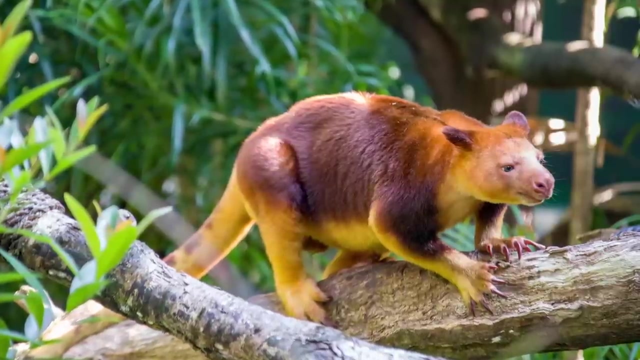 australia's mount kosciusko, which stands at just over two thousand meters. at almost 800,000 square kilometres, New Guinea is the world's second largest island and features many curious animals, including a particularly interesting marsupial, the Goodfellow's tree kangaroo. These furry fellows weigh around seven and a half. 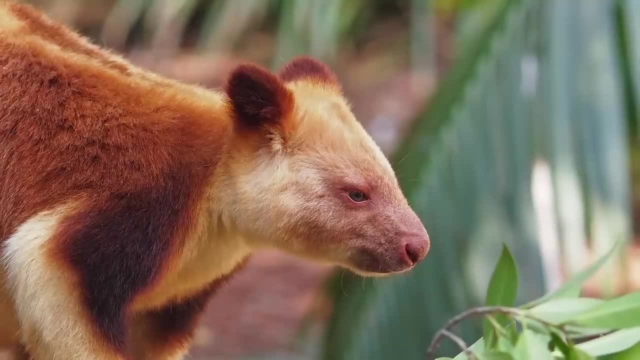 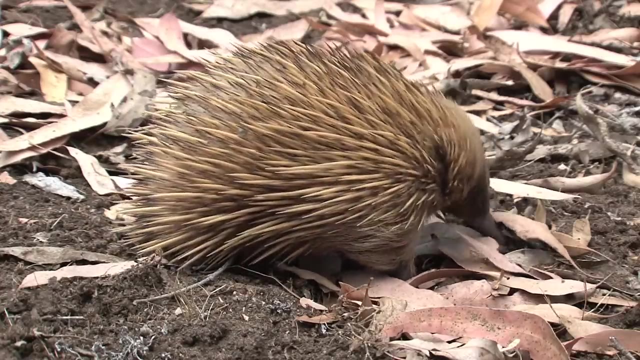 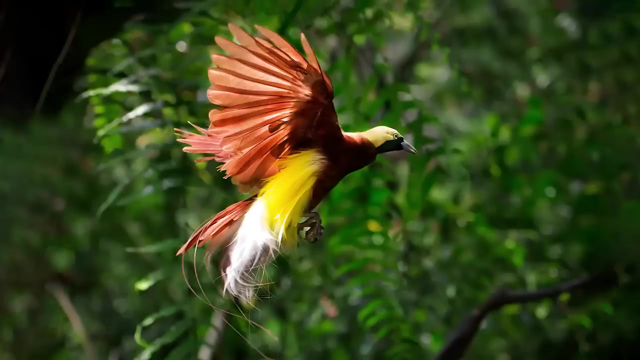 kilograms and, unlike their Australian counterparts, have brown and cream fur. The long-beaked echidna is a prime example of a monotreen mammal that exists in this realm and comes very close to, but does not cross, the Wallace line. The birds of this island are many and include a particularly exotic. 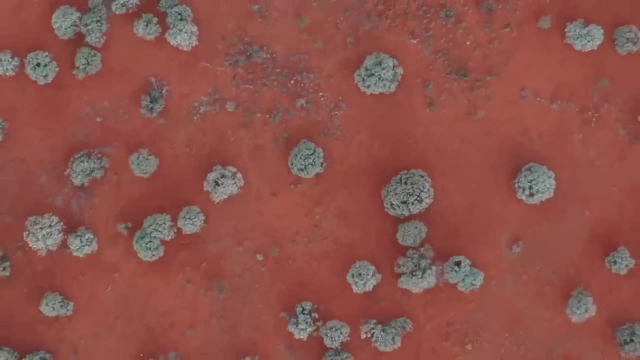 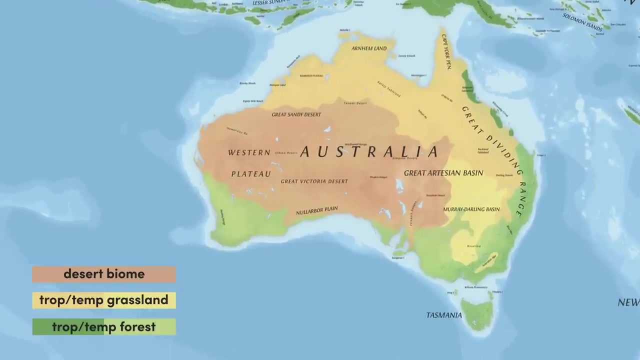 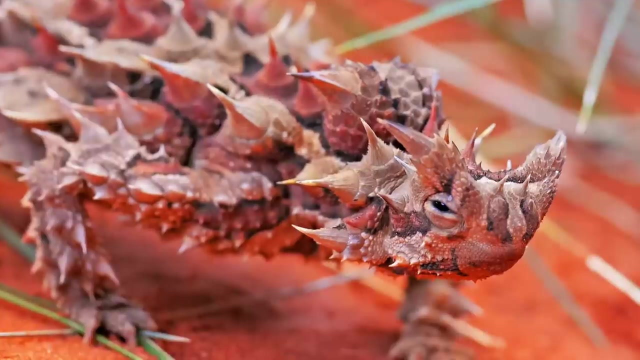 family, known as birds of paradise. Australia is the world's sixth largest country and features a variety of biomes. The central and western portion of the country is dominated by areas that receive very little precipitation and are therefore classified as desert. The thorny devil is endemic to Australia and 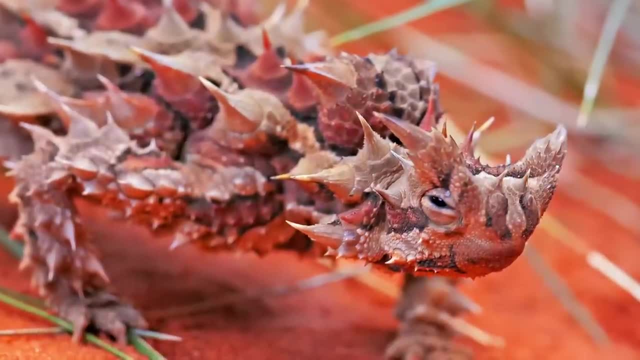 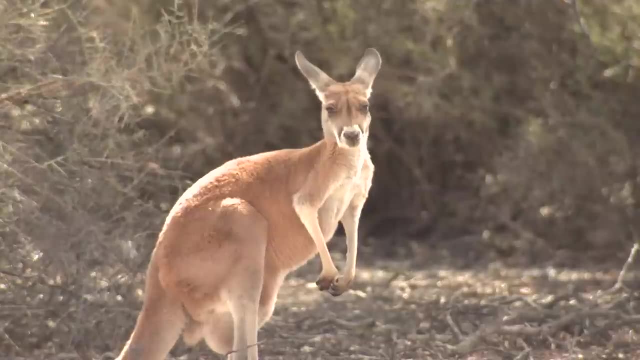 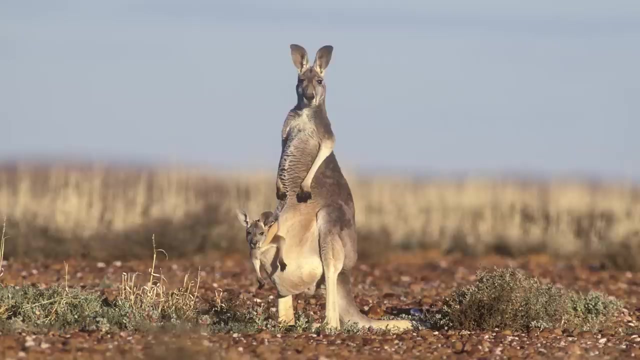 in addition to its thorny exterior and intricate camouflage, exhibits a fake head on the back of its neck. Australia's red kangaroo is the largest of Australia's many marsupials and varies in color between sexes. Males are brick red, whereas females are grey. The eastern- 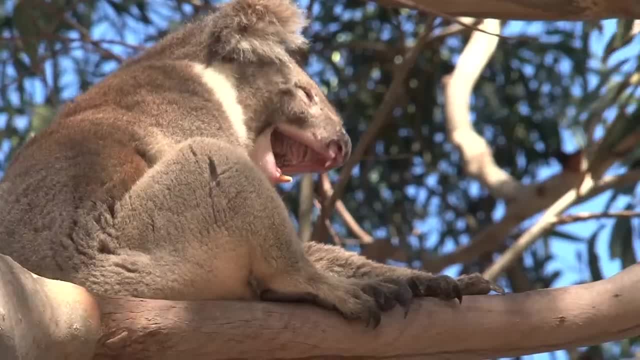 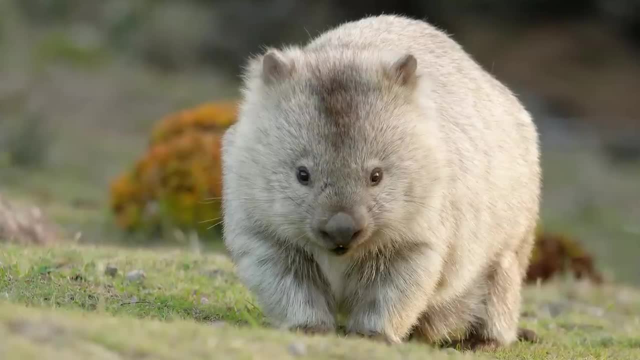 portion of this country is made up of grassland and forest. Here, koalas can be found traversing the treetops overseeing wombats, another marsupial who live in underground burrow systems. Australia is, of course, famous for its snakes and 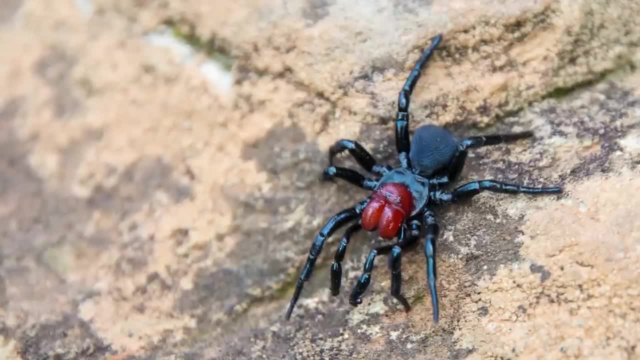 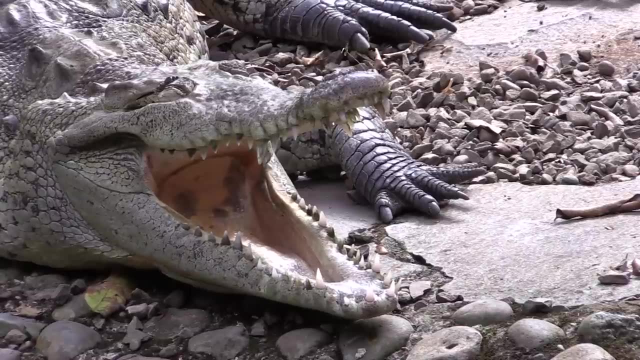 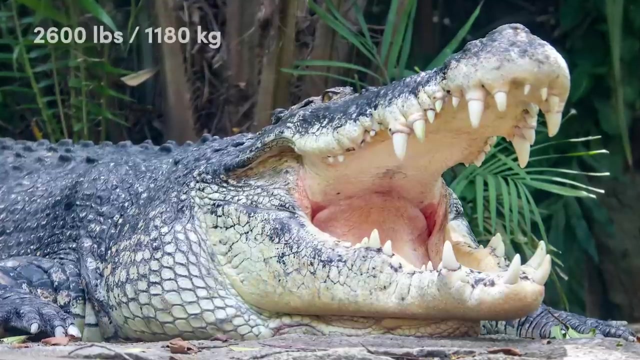 spiders. One of the most striking arachnids is the red-headed mouse spider, with males exhibiting a red head and jaws. It would be a travesty to discuss Australia without exploring its waterways and ocean. The saltwater crocodile is the largest reptile on earth, weighing north of 2,600 pounds. They exist on 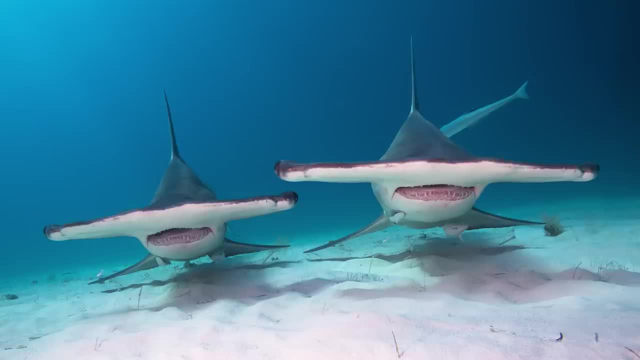 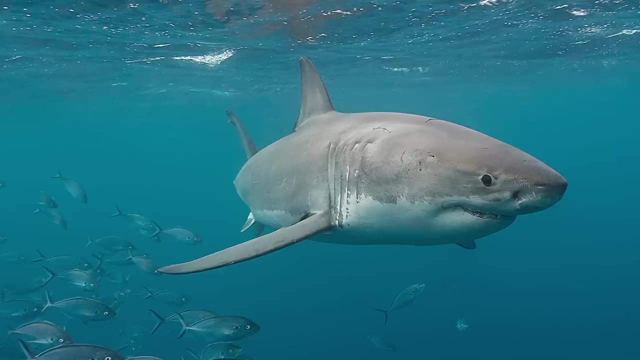 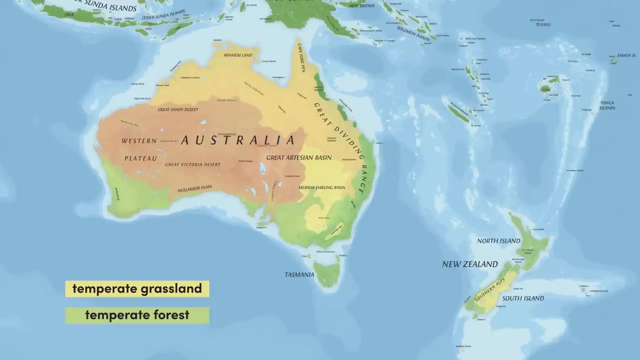 Australia's northern coastline and into Southeast Asia. The species of shark in these waters are numerous and range from hammerheads and tiger sharks to the infamous but beautiful great white. New Zealand is found southeast of Australia and, although it is in the same realm, is home to quite a different array of. 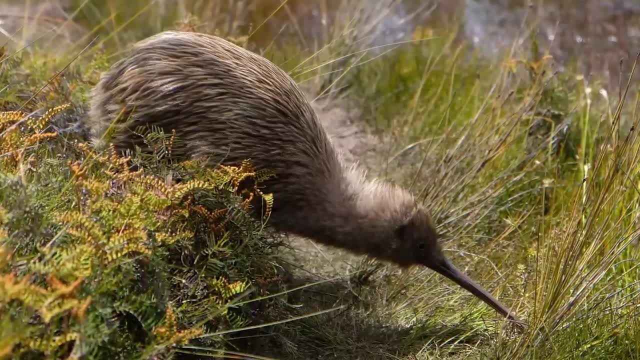 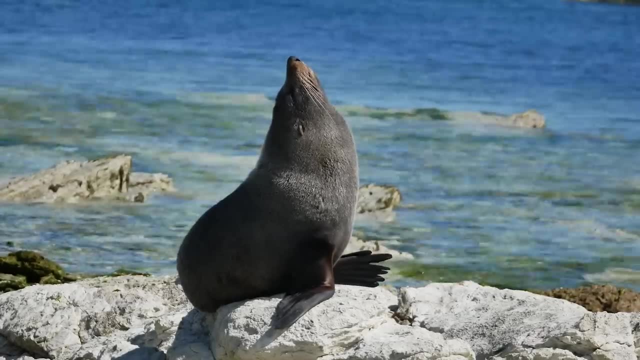 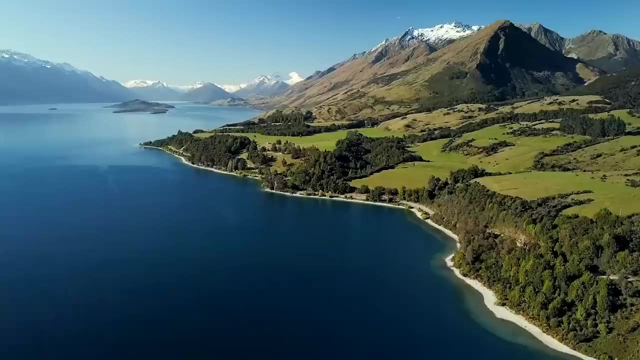 animals, The most iconic by far is the Kiwi, after which the humans of these islands are nicknamed. Mammals of the marine persuasion include various types of pinniped, such as the New Zealand fur seal, and whales such as the Hector's dolphin, which has a unique coloration. Interestingly, there are no marsupials or 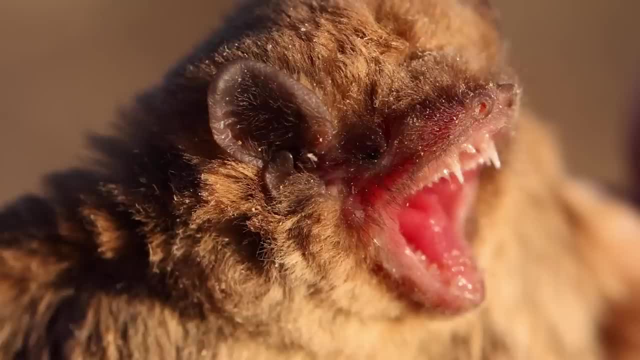 monotremes here. They are only found in the southern parts of the world. The most popular of these animals can be either a mussel that lives in the ocean or a hot 그렇. In fact, bats or peck a pecker and Maori are the nations. 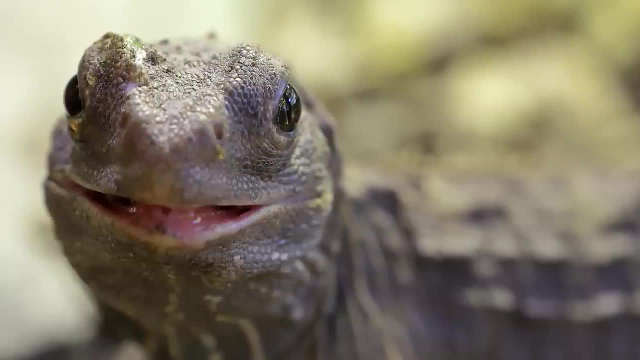 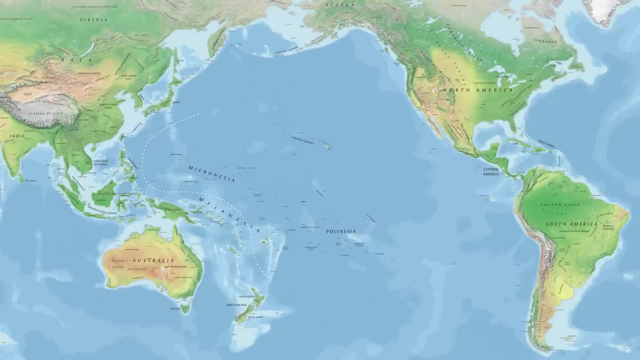 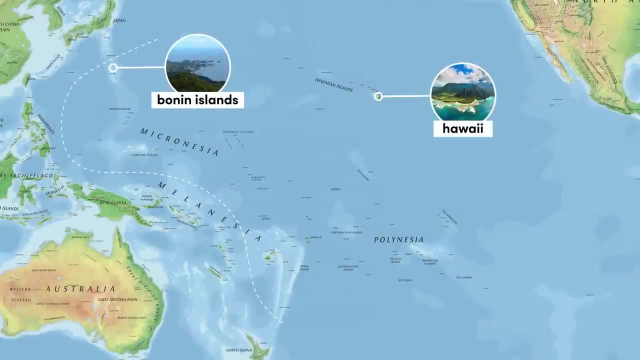 only native land mammals Representing the reptiles of New Zealand is the tuatara, a rare species found on the North Island and the very northern tip of the South Island. The oceanian realm is made up solely of islands in the Pacific Ocean, stretching from Japan's Bonin Islands and Hawaii in the north to. As such, it is the smallest realm on Earth by landmass. The topography here is limited due to the size of the landmass, but the highest peak in Hawaii still reaches over 4,000 meters. Migration to and from these islands is limited for land mammals due to the long, treacherous